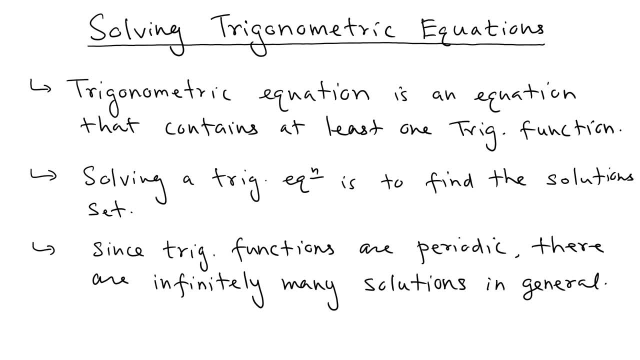 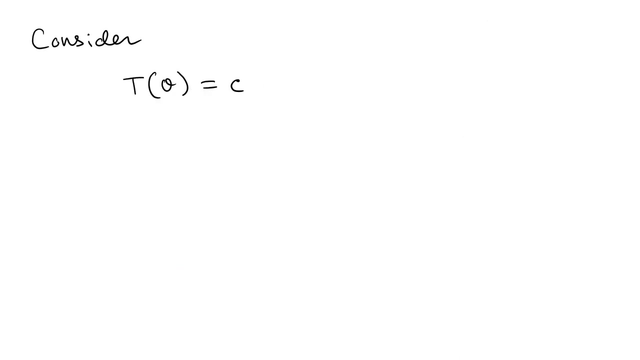 So there's a one major difference between trigonometric equations and other equations. We know that trigonometric equations are periodic functions. So trigonometric functions are periodic. Since the trigonometric functions are periodic, so there are infinitely many solutions for certain equations. So that's like a very different situation compared to polynomials and other equations. We don't know that when polynomials, if a degree n polynomial, there can be at most n solutions. But that's not like this here. So when you have trigonometric equations, you have infinitely many solutions for certain problems depending on the value that we're going to pick. So in general. So let's look at a certain situation. Let's say we have a general equation t theta equal c, where t theta is like any trigonometric equation. So we have a general equation t theta equal c, where t theta is like any trigonometric equation. So t theta is like any trigonometric function. So t theta is like any trigonometric function. 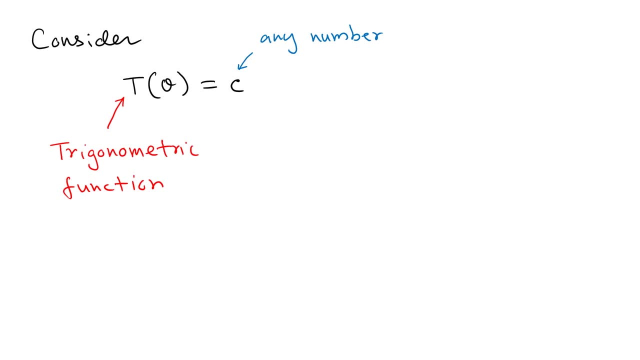 c is any constant. So for example, let's say, let's look at this situation. We have sine theta equals c. So that means sine theta equals a constant. So we know that the sine graph has this format. So it's going to start with 0. So let's say we just look at one period. So 0, pi, and 2 pi. And then we know that that's going to go with two specific values, 1 and negative n. Now, let's see several situations. For example, let's say you're going to pick a c value 1 half. So if you pick a c value 1 half, that means we're going to find for what theta this function equal to 1 half. So for example, so in geometry, what we can do is we can draw a line up through 1. 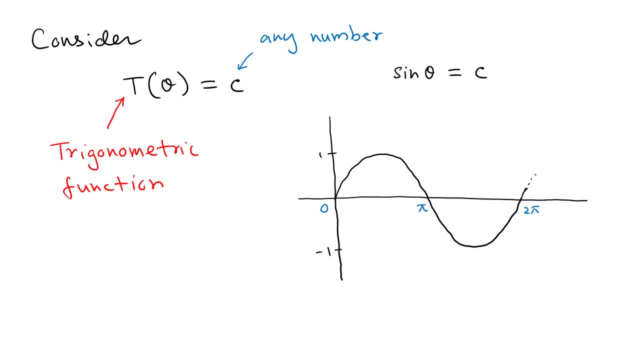 1 half. So we can draw a line through 1 half. And then look for what values are going to give you that value. You can see, for example, in this case, so we can map that value back to the x variable, back to the x variable. So when you do that, you can see, so this is, there's a 1 value here. And there's also another value there. So you can see in this special value 1 half, in this special value 1 half, there are two values. 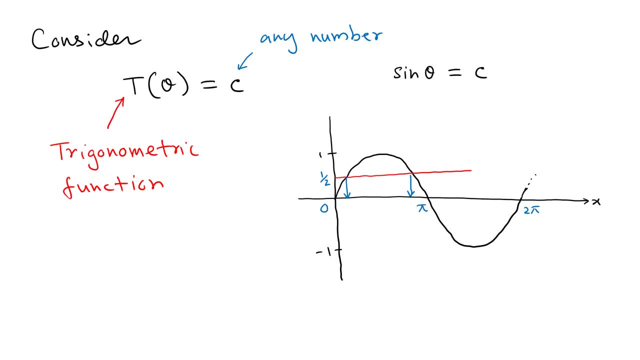 So you know that from the sine function, so for example, if you have, so I'm going to call the first value is x1 and the second value is x2. So you can actually find those two values. For example, we know that the x1 is simply pi over 6 or in degrees, it is 30 degrees. And then there's another value x2, which is 150. So you know those two values. So that means even like if you pick 1 half, you can see there are two values there. So for example, let's see like another value. 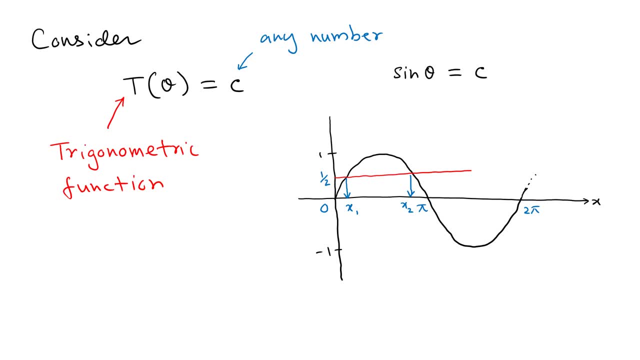 For example, let's say 1. So if you pick 1, so you can see in this case, there's only one value. 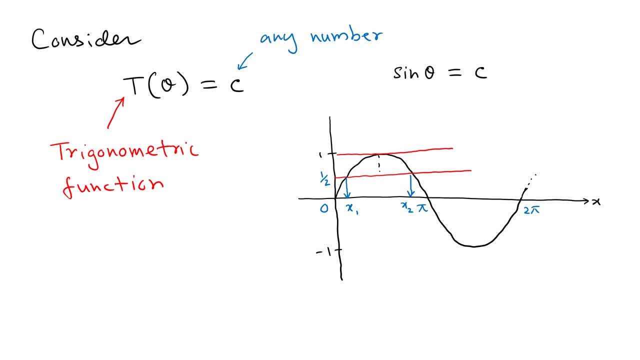 So in this case, you don't have two values. You can see there's only one value. So that's the value. 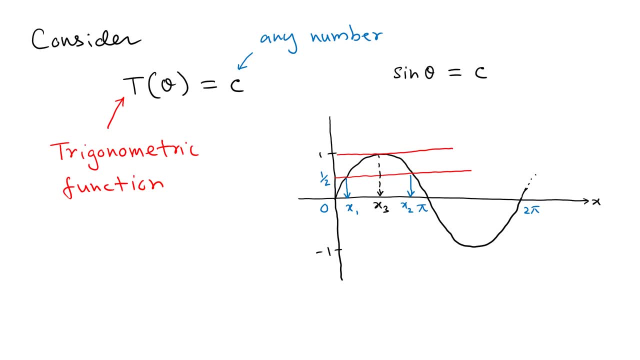 I'm going to call x3 in this one period. So you can consider just one period from 0 to pi. And you can see that there's only one value in this case. So that means if you pick c as 1, so this is the c equal 1 situation. This is c equal 1. So you can see that there's only one value in this case. So that is equal 1 half situation. So for c equal 1 half, you have two values. For c equal 1, you have one value. And also the same thing, like for example, let's say you pick negative 1 half. So you pick negative 1 half, and you can see it again cuts at more than one point. And then those two values are going to map to two values. So there's one value here. And also, there's another value over there. So there are two values again. 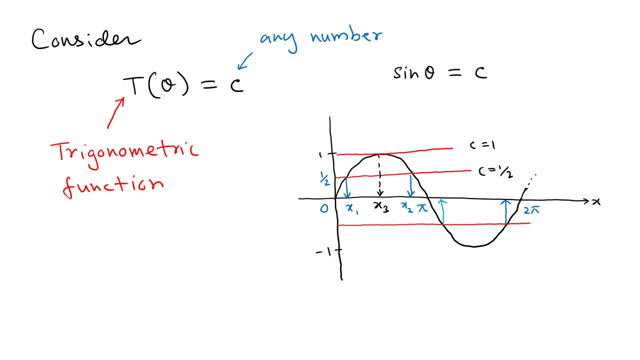 So we're going to pick a value like up here, like 3, like 2, let's say in this case 2. So if you pick a value 2, and you can see that this graph never crossed this value. So that means if you pick a value 2, what happens? There are no solutions. So that means there are several cases here. So you can see if you have 1 half, you have two values. If you pick c equal 1, you have one value. If you pick like c equal 2, you can see that there are no values. So that means anything, those three values are going to be in a situation like this, especially in one period 0 to 2 pi. And then since it is periodic, what we can do is simply adding 2 pi, you can generate, adding or subtracting multiples of 2 pi, you can generate all the other values. So that is what we're going to do in general. We're going to find the values from 0 to 2 pi or 0 to 360 in degrees. And then we're going to add multiples of 2 pi or multiples of 360 degrees to find all the other values. 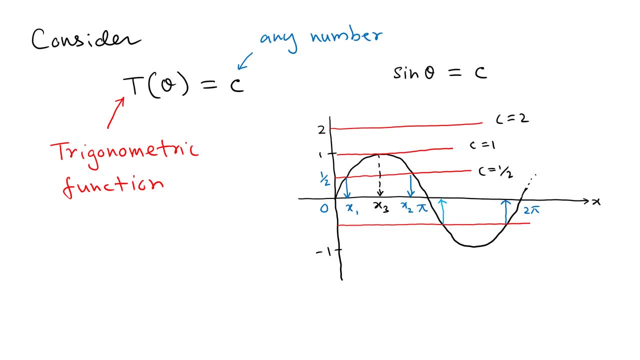 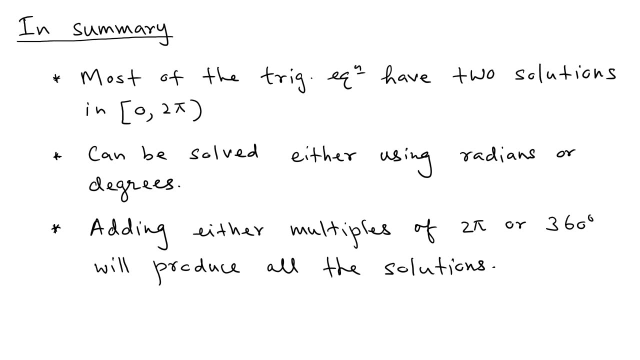 That's what we do in general. So we can summarize this result like this. So you can see that in most of the trigonometric equations, so there are two solutions. There are two solutions in 0 to pi or 0 to, or you can say 0 to 360, depending on whether you want to do it in degrees or you want to do it in radian. And then, and it can also be done in degrees. So you can do it in degrees or you want to do it in radian. And then, and it can also be done in degrees. So you can do it in degrees. So you can be solved in either radian or degrees, depending on the need. And also adding either multiples of 2 pi or 360, again, depending on radian degrees, you can find all the solutions. Here, multiple means integer multiples. You have to be careful with that, integer multiples, not any multiple. Integer multiples, adding integer multiples of 2 pi or 360, you can find all the solutions. 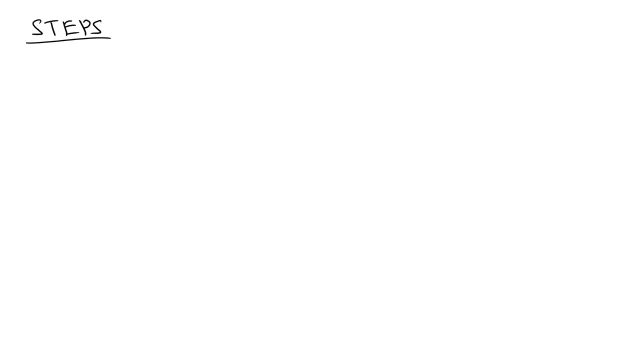 So a general problem has five steps. So let's look at those two steps. So what we normally do is if we get a problem like that, what we do is we factor. And then after we factor, we can set each factor equal to 0. And after that, we can isolate. So we can set each factor equal to 0 and isolate the trigonometric functions. So sometimes what happens is those trigonometric functions are like we normally try to bring it to sine, cosine, and tangent. If it is not sine, cosine, tangent, we try to rewrite. So let's say you have secant or cosecant, secant, or cotangent. What we're trying to do is we're going to convert them into sine, cosine, tangent. So that's what we do at the beginning. But this is not a must. But this is going to make it easy to solve if you are familiar with those values. But you can still simply solve using cosecant or secant. But we normally don't do that. We just try to bring it to sine, cosine, tangent before we solve. 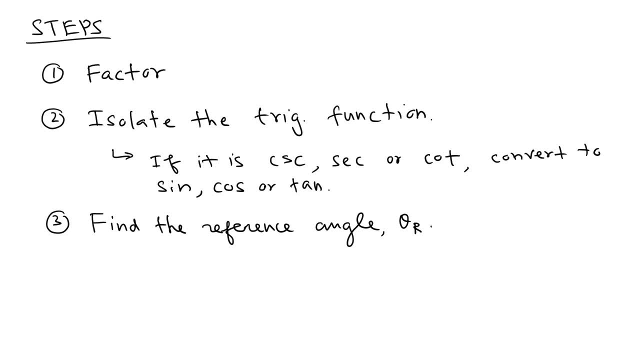 So the third step is... after we isolate the term, we're going to find the reference angle. We're going to find the reference angle because reference angle method is the easiest and straightforward method. So we're going to find the reference angle after we isolate the trigonometric function. And then what we're going to do, we're going to find the principal values. So what are the principal values? And you can see in the discussion earlier, when you draw the line, it's going to cut at two points. You're going to find two values in the domain that are going to give you the value you need. There are two solutions or sometimes there are one solutions. Those are in 0 to 2 pi. Those are we normally call principal values. So you'll find the principal values first. 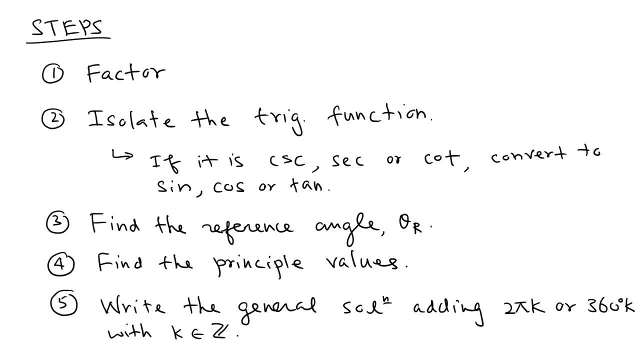 And after you find the principal values, what you can do, you just add the multiples of like multiples of 2 pi or you simply add 2 pi k or 360 k where k is an integer to find the general solution. So these are the five steps method to solve a general trigonometric equation. 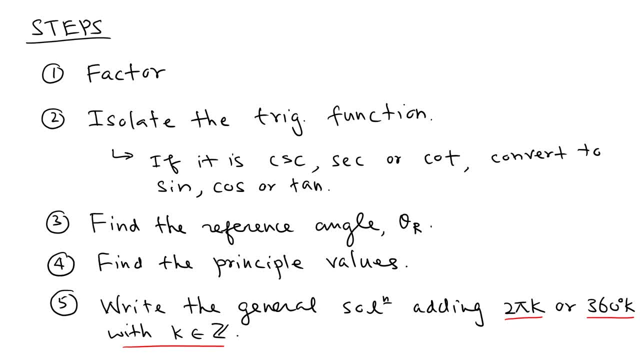 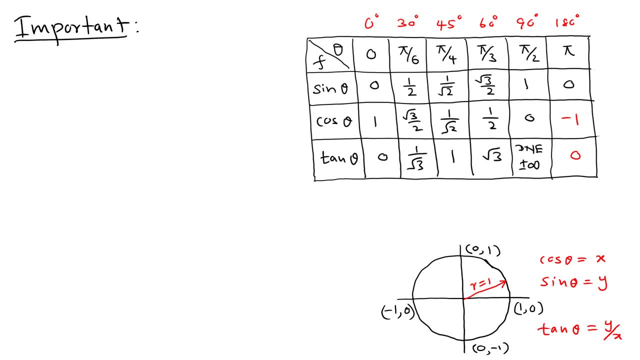 Also there's a major help or tool that we normally use. So this is the general formula. So like let's say for example, if you have f theta equal like you're going to, what we normally do, like if you have function trigonometric functions, we normally write this one as, so you can always write this one as plus or minus f the reference angles. That's the trick. So what we normally use here and you can see that the other the sign, the sign we're going to find using the ASTC argument so that we discussed earlier. So ASTC argument going to give you the sign and then to find the function trigonometric function value at the reference angle, we're going to use the table on the right. So this is this part simply coming from the table. And also this table is the common table. 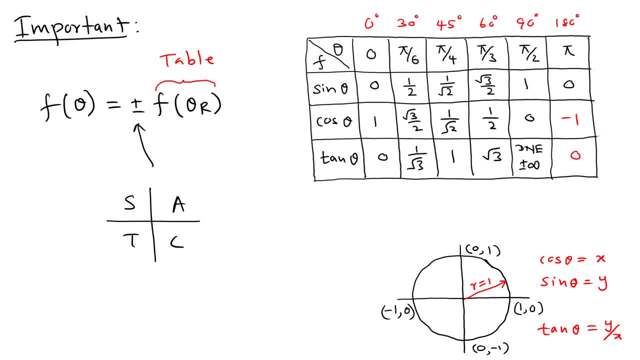 So you can see that the one trigonometric values that we normally use and then you can see that, so there are certain patterns here, like for example, if you reverse the values in the sign, you're going to get the values in the cosine. That's one of the common practice and also you can see that to get the sign values, what you normally do is you're going to write 0 1 2 3 and 4. by 4 we divide each number by 4 so write 0 to 4 divide by 4 and take the square root once you do that you can see that these are the values uh in the sine table so you can see these are exactly the values in the sine table uh from 0 to uh 90 degrees and then to get the cosine values you reverse the order so this this is the trick you can use uh you write 0 to 1 2 3 4 and then divide by 4 and take the square root and then uh to find the values for multiples of pi over 2 to find the values of multiple of pi over 2 we use the unit circle so uh so use the uh unit circle so that's what uh those are the common 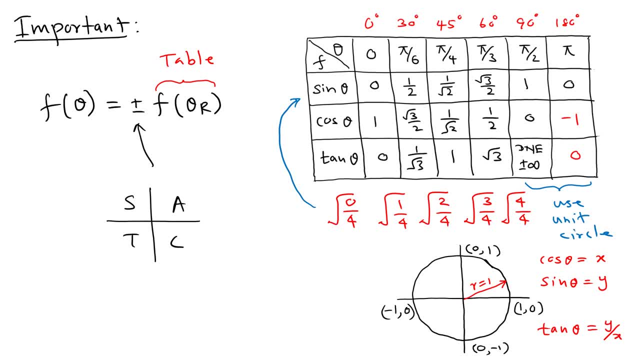 things that we use so unit circle means the circle with the radius of 1 and then you can see that the cosine is the x coordinate sine is the y coordinate tan is the uh the uh 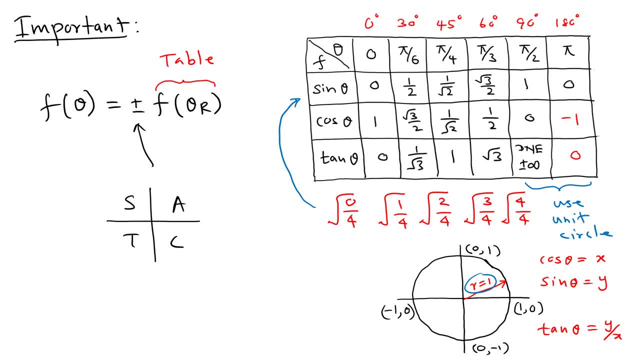 the diff you can divide the the quotient of the y coordinate or x coordinate um if it is defined so you can see you can find all the values using this so these are the things that you need to remember and you can see using these you can easily solve any problem of this type uh so let's also look at the quadrant 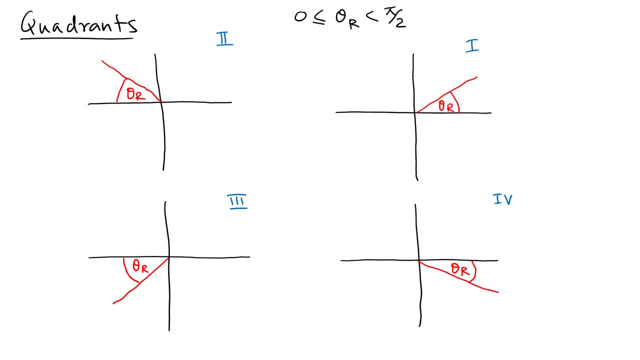 what happened in the quadrant so um uh so to find the reference angle so let's say so these are the reference angles so the question is if you know the reference angle how to find the angle so for example um so you can see that uh in the first quadrant so the angle is simply theta r and then you can add multiples of um 2 pi but here just i'm going to rise in the principal values and then here you 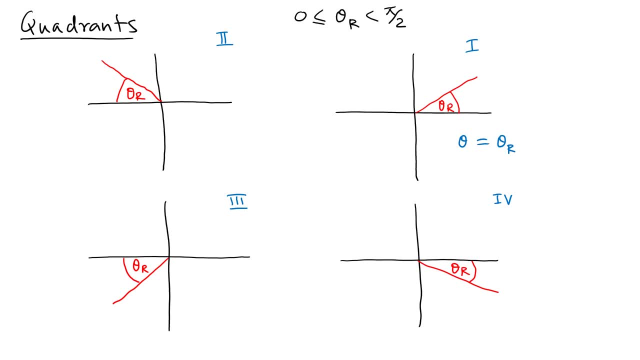 can see the principal value is simply so uh so 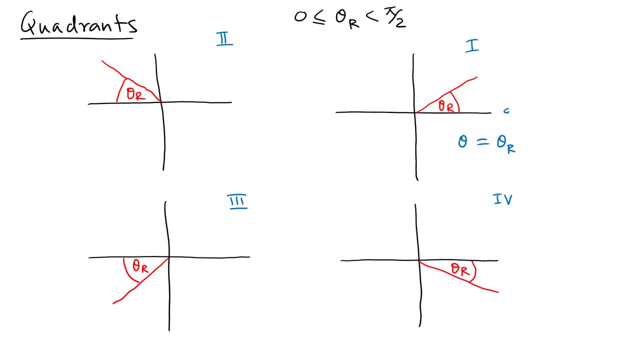 this is this is the zero and then this is uh we normally write this as pi this is also pi this is 2 pi. 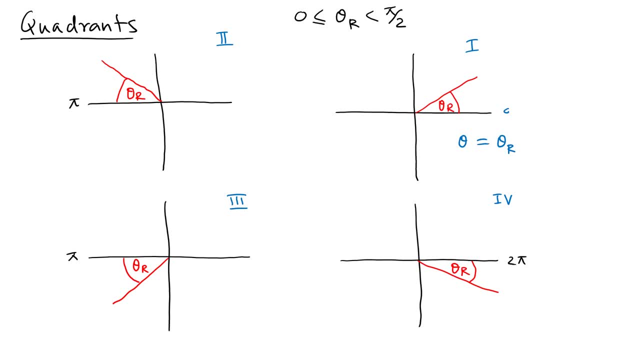 so you can see um for at this time in the quadrant two your value is simply theta equal pi minus the reference angle 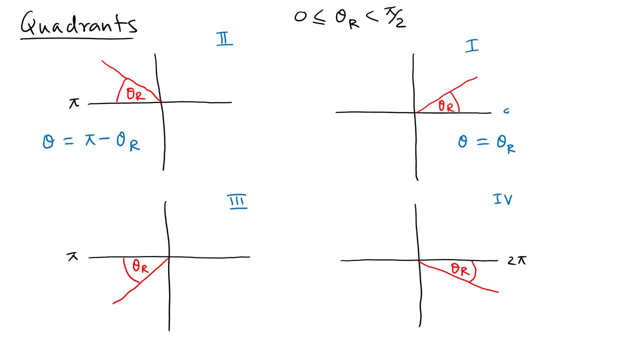 that's what happened for the quadrant two for the quadrant three you can see that theta is simply pi plus the reference angle for the quadrant three because of pi and a little bit more than 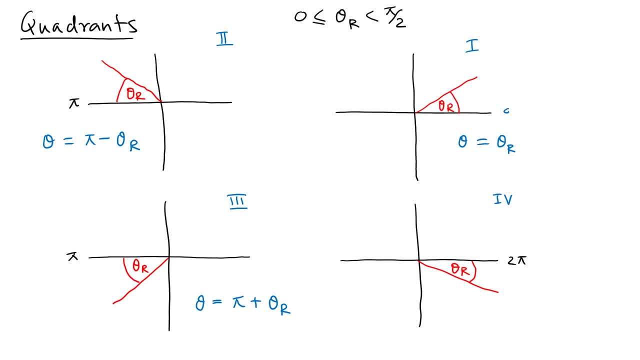 uh like pi plus theta r theta r the reference angle and for the quadrant four you can see it is uh 2 pi minus 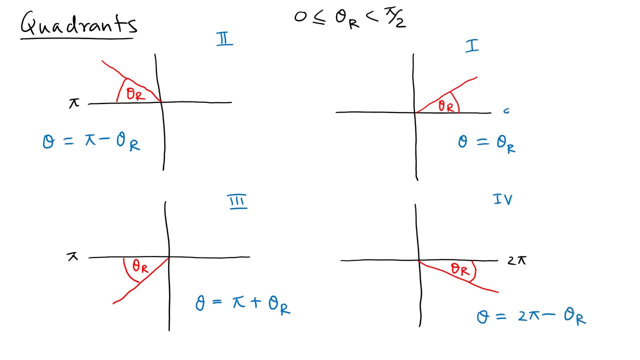 the reference angle so those are the three cases and you can see that we can use this a lot depending on the situation and these are the principal values to get the other values what we normally do we can add 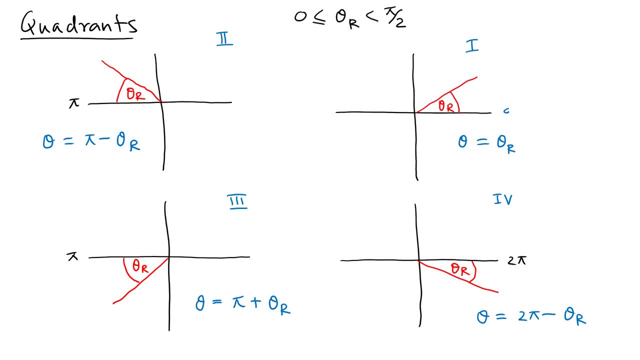 multiples of 2 pi or multiples of 360 um depending on the radian or degrees that we work with 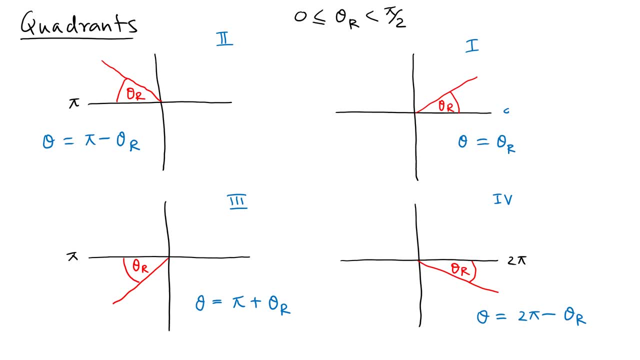 so let's try to look at several problems now 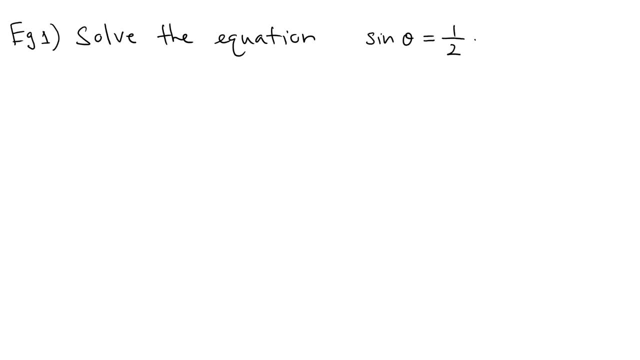 so as the first problem are we going to solve sine theta equal one half so uh so let's look at the corresponding graph in this case and you can understand what's really going on here so um so the sine graph uh we're gonna look at just the first period so so this is the sine graph and this is the same situation we discussed uh at the beginning so we can see that this is zero and then pi and two pi the first period and then uh we're gonna look at the values so we're gonna draw the line uh one half and then you can see there are two values there's a one value here the other value there so there are two values so uh what we are going to do is we're going to find the reference angle first and then also you can see that um we're going to find the reference angle first and then also you can see that this is a sine and this is positive so that means 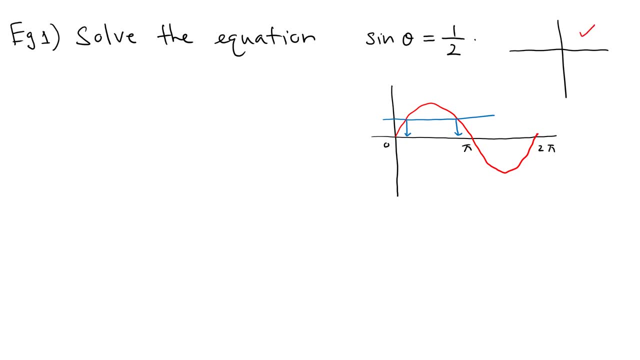 the angle should be either in the first quadrant or the um second quadrant due to the astc argument 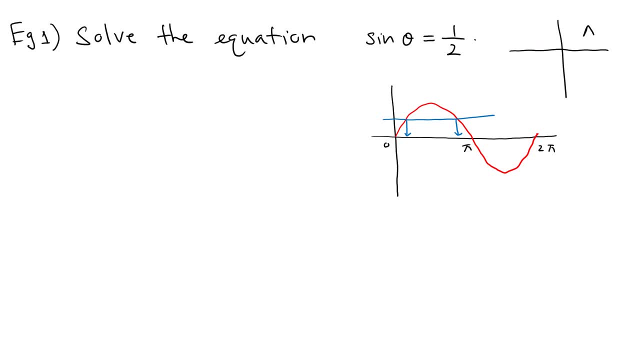 uh so if you write it back so this is a s 3 c that means uh it is positive in the first quadrant or sine is positive in the first quadrant or the second quadrant and then you can clearly see that that's that's exactly what happened so what we are going to do is we're going 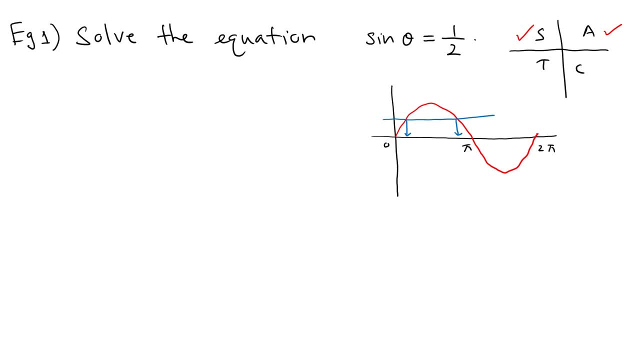 to uh normally do is um we're going to find the so if you get a problem like that what we normally do is we're going to find the reference angle first so that means theta r so uh so what is theta r theta r is 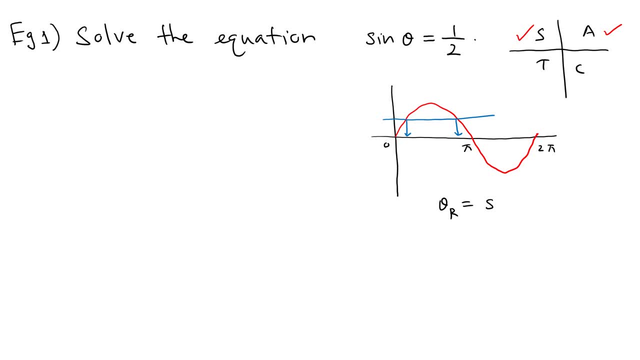 we ignore the sine we can write sine inverse one half so we write and then from the common table we know that the uh for theta equal pi over six for theta equal pi over six uh we get one half so i mean that's the reference angle since you know the 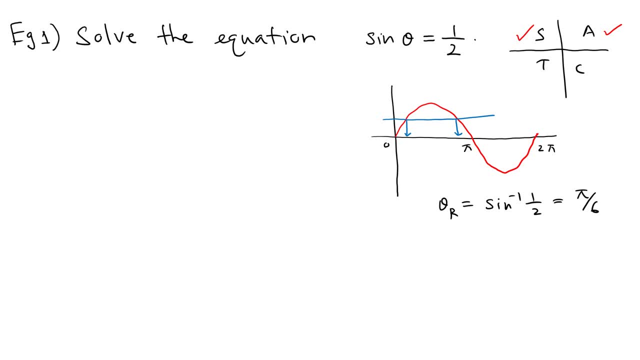 reference angle that means your values uh one value is pi over six to find other value you can see uh to get the other value what we need to do is you can subtract because you can see those those gaps are the same so these two gaps are the same you can see this gap and that gap are the same that means you have to subtract this value so that means this one second value it should be pi minus pi over six because the gaps are the same and also we discussed this in uh just a minute ago if you look at the four quadrant in the second if you need the value if you need to find a value in the second quadrant what we normally do is pi minus the reference angle pi minus the reference angle okay so uh so that's exactly what happened uh in this case uh so we can also see this in a um in the quadrant setting so these are the uh the quadrant and then you can see so that is in the first quadrant 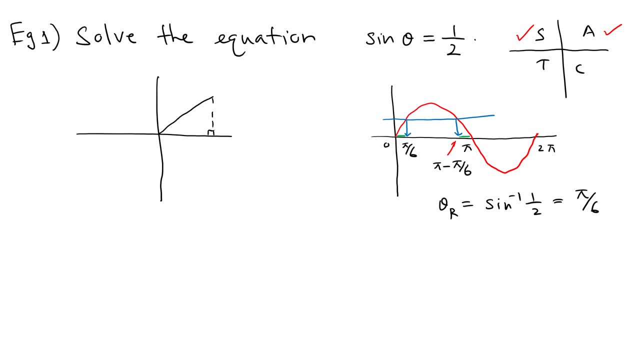 so this is the uh the value uh pi over six and this is uh opposite over hypotenuse and then the value in the uh second quadrant and you can draw it like that 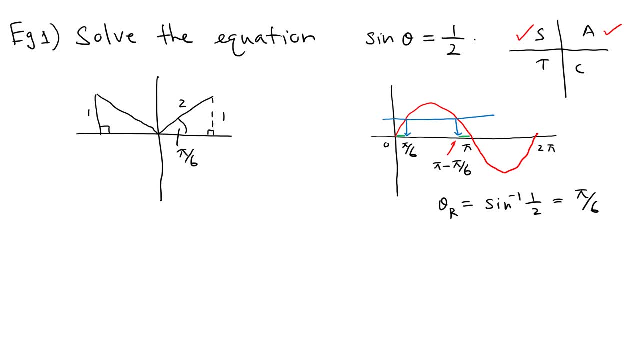 so you can see it's also positive that means these are y coordinates positive and then this is the hypotenuse so we have we have that and then you can see this is again the 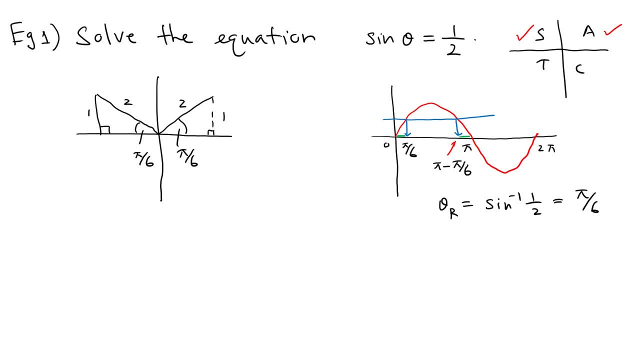 same uh reference angle pi over six so to find the angle what we do so that's the angle we are looking for 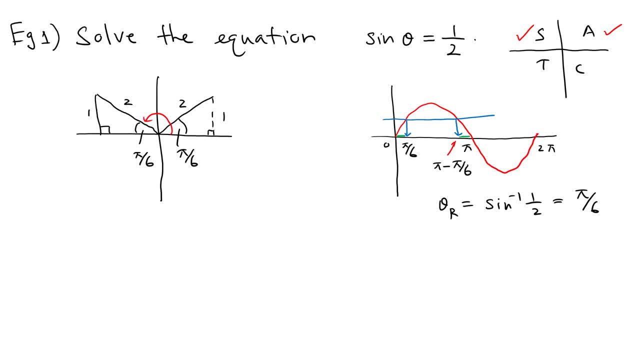 to find the angle what we do it is pi minus because this angle is a pi straight angle so we're going to pi minus pi over six so that means you can write the solutions uh like this 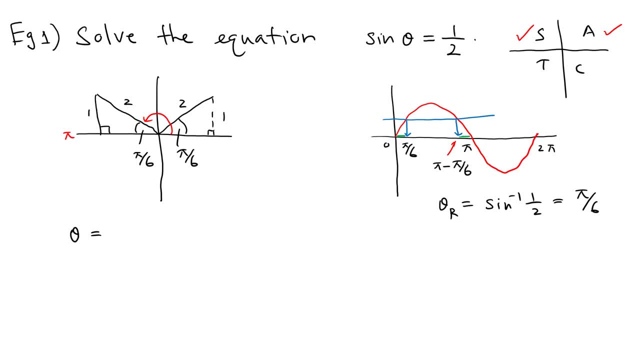 so we can say theta is uh pi over six that's the one in the first quadrant 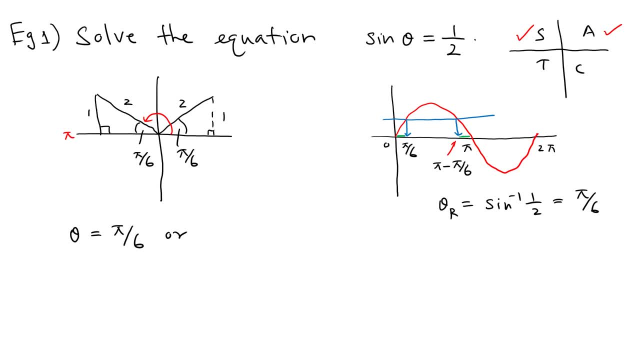 or to find the value in the second quadrant or theta equal pi minus the reference angle that's always the case 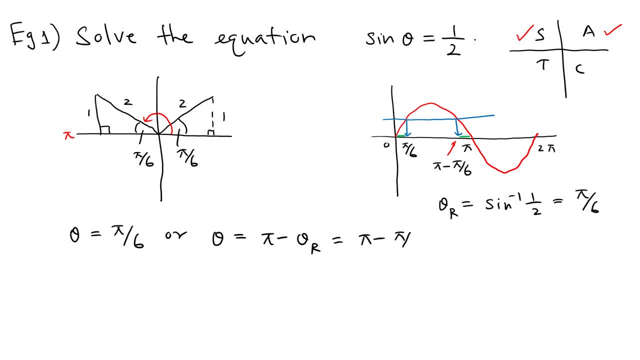 so that means it is pi minus pi over six reference angle does not change so if you simplify you can see this is simply uh five pi over six taking the common denominator so this is in the quad uh in zero to two pi there are no other values those are the only values you're going to get from zero to pi 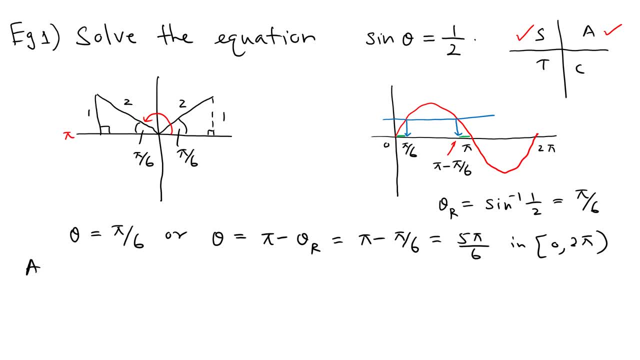 so we are going to run a solution using this so we can say eta is equal to plus continuous 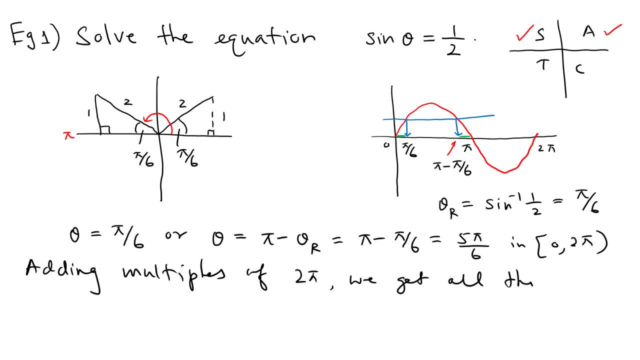 2 pi because the 0 2 pi 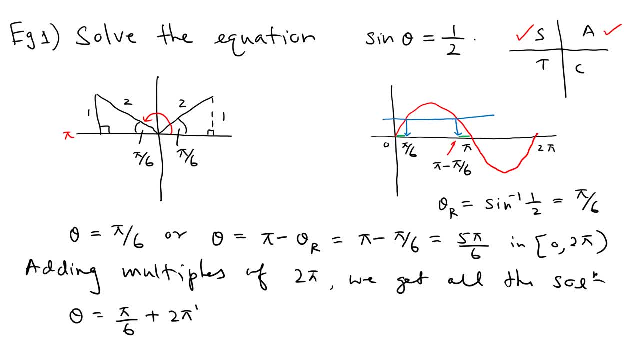 2 pi now what we can do adding multiples of 2 pi adding because you can see it's periodic that means if you add a 2 pi 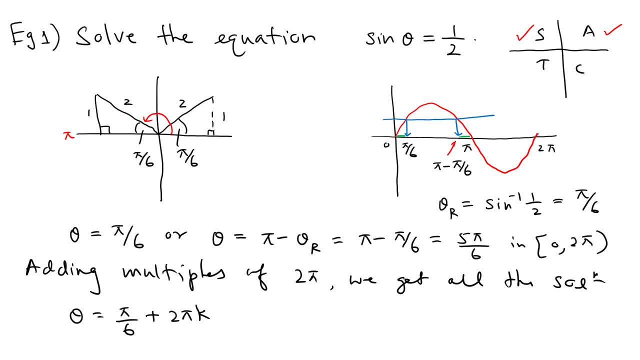 you get the same sign or um you can see the other value is 5 pi over 6 plus 2 pi k so you can see where 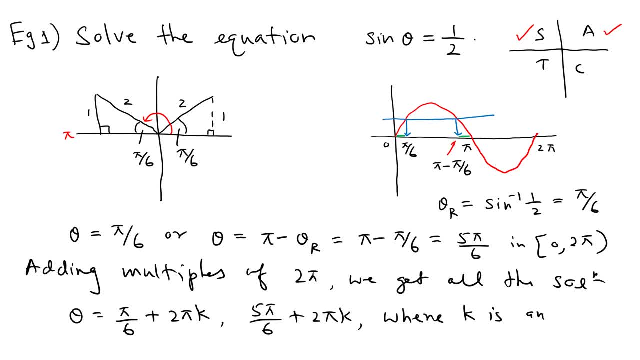 k is an integer where k is an integer so it's integer multiple of 2 pi that's how we did we add integer multiple of 2 pi 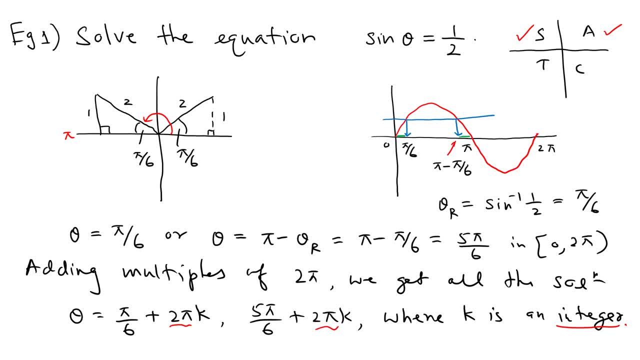 so this can give you all the solutions of this equation so this is how you solve the first equation 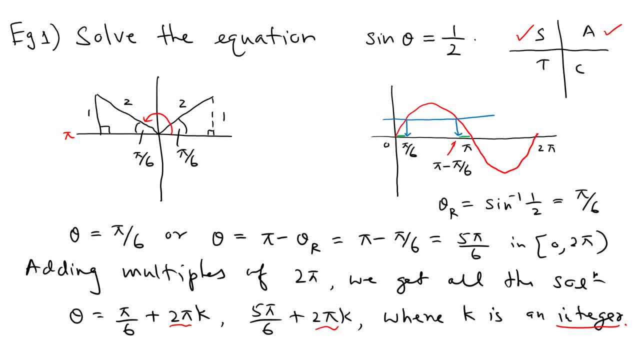 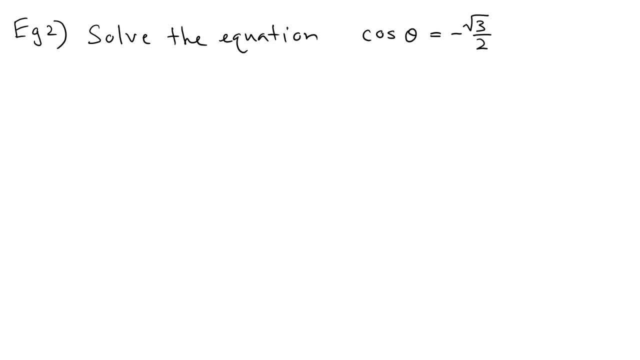 so let's look at the next one as the next problem are we going to solve cosine theta equals negative square root 3 over 2 and you can see that square root 3 over 2 is a common value that you can find on the table and also we see that there's a negative sign here so that means if you have a negative sign here you have a negative sign here so that means according to astc 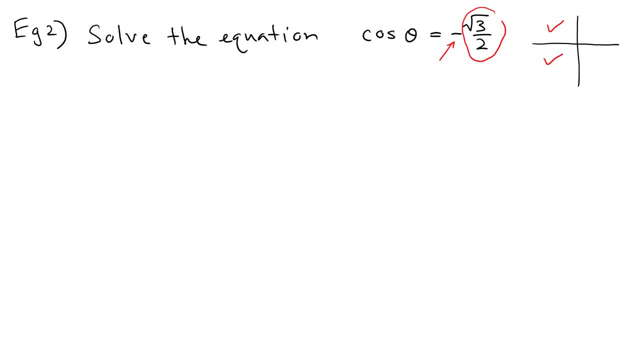 this angle has to be in either in the second quadrant or the third quadrant and that means if you know the reference angle one angle has to be pi minus a theta r the other one has to be pi plus theta so that means your goal is to find the reference angle first 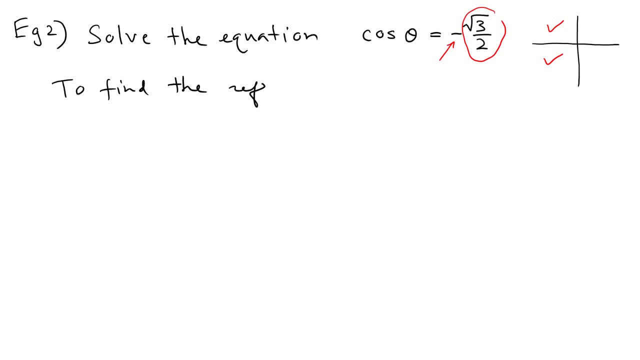 so to find the reference angle to find the reference angle what we're going to do are we going to ignore the negative sign and we're going to say theta r is equal to cosine inverse i square root 3 over 2 this is what we always do we ignore the negative sign and find it so this is simply coming from the table so using the table and you can see that this value is is a cosine um pi over 3 so is cosine inverse i square root 3 over 2 that means this is simply pi over 6 so that is the negative sign so this is a a reference angle so once you know the reference angle then you can uh draw the situation this is like optional but it's gonna clear uh what's going on here so um so this is the uh second quadrant and then uh that's the perpendicular and this is uh pi over six that's the reference angle so that means this is the uh first theta one uh and then uh for the third quadrant and you can see the reference angle is still the same 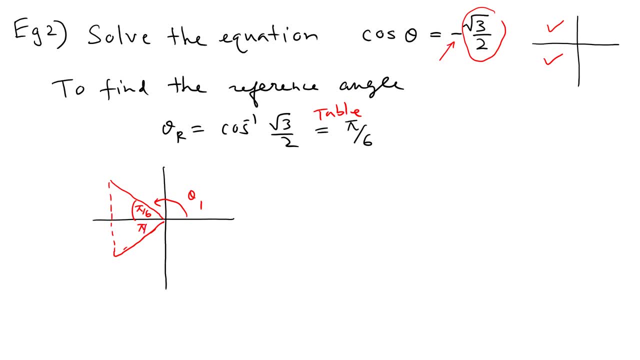 so it doesn't change so this is again uh pi over six so this is the uh other angle so you can write it uh like this that's the second angle so uh so in this case you can write 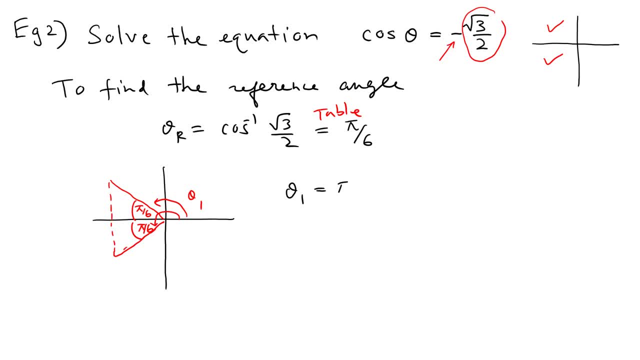 theta 1 which is simply pi minus the reference angle so that means pi minus pi over 6 so taking the common denominator multiplying by 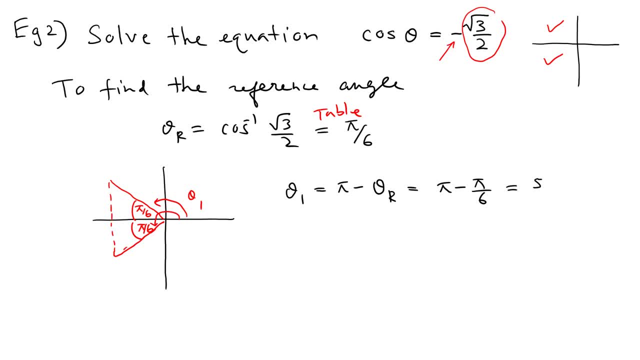 are top and bottom you can get simply 5 pi minus 6 as the first angle for the second angle what we're going to do it is pi 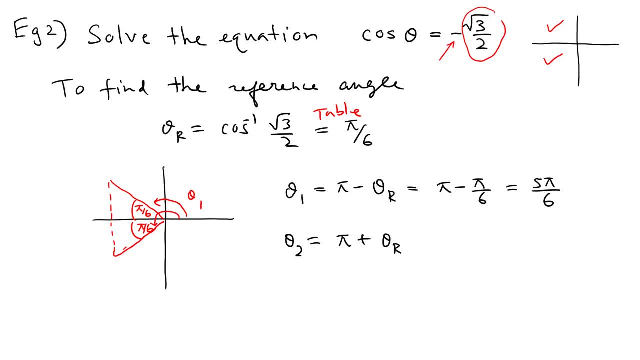 plus the reference angle so this is again pi plus pi over 6 again multiplied by 6 and 6 you're going to get this is 7 pi over 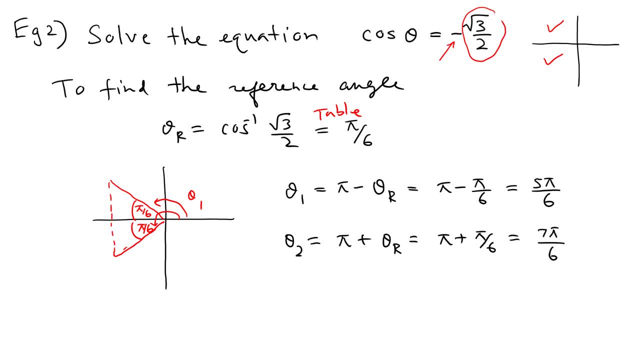 6. so those are the two are principal angles so that means the solutions are so the solutions are so you can simply write theta are equal 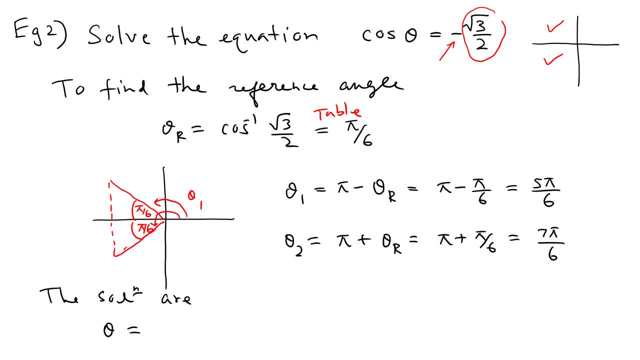 theta equal the first one is um so you can see that it is 5 pi over 6 plus 2 pi k comma the other one is 7 pi over 6 plus 2 pi k area 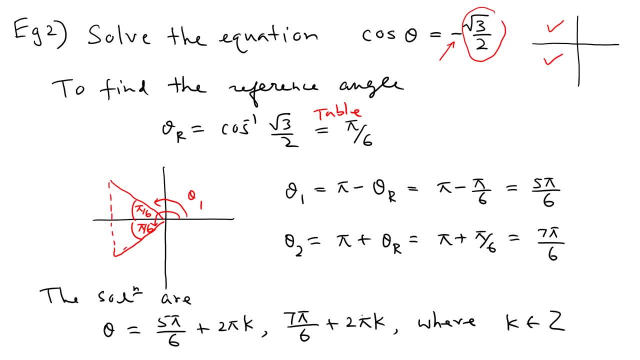 k is an integer so you can write it like that k belongs to set of integers so that is how you write the how you solve the equation so let's go to the next one that's the next one we're going to solve 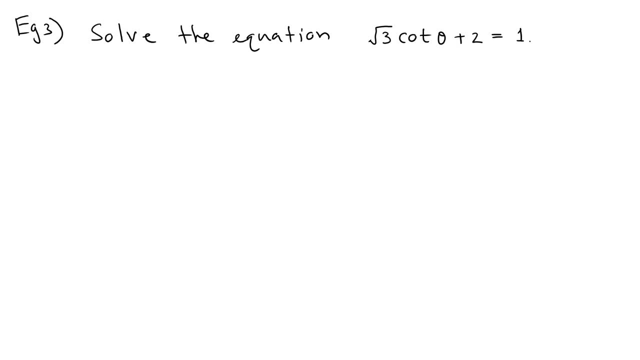 this problem and we have square root 3 cotangent theta plus 2 equal 1. so there are a few things that we need to solve 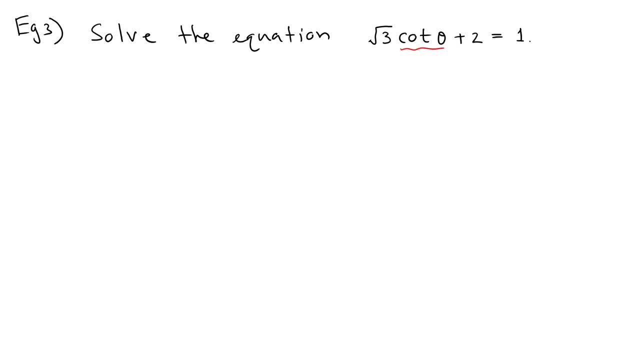 that we need to focus on and you can see that this is not a sine cosine or tangent that means it would be better to convert this into one of those that's that's one thing and also since we solved the first two problems using radian are we going to solve this problem in degree it's not a must but let's see how 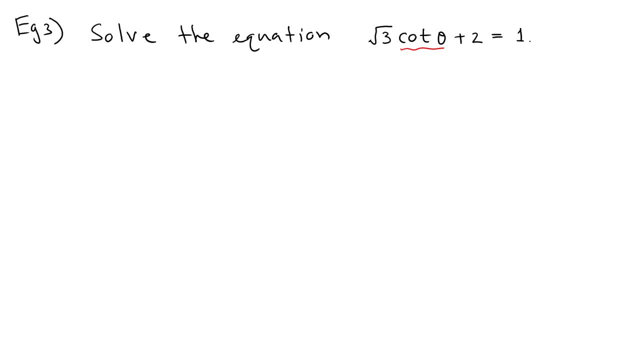 we can solve the problem in degrees so we're going to see two things now so we can start with the problem and we can see we have square root 3 cotangent theta plus 2 equal 1. so we can isolate the co-tangent term first so to do that first we move 2 to the other side and then are we going to divide by square root 3 so we're going to move the 2 to the other side so that means going to be 1 minus 2 that means going to be negative 1 and then are we going to divide by square root 3 so that means cotangent theta equal negative one over square root damage theta so and then we know that one of the fact uh the tan theta is 1 over cotangent theta and then cotangent theta is 1 over tan theta that means uh if you flip this equation up if you make it upside down you're going to get the you can you can make this uh tangent so so we're going to flip this so that means once you flip it you can write this one as tan theta 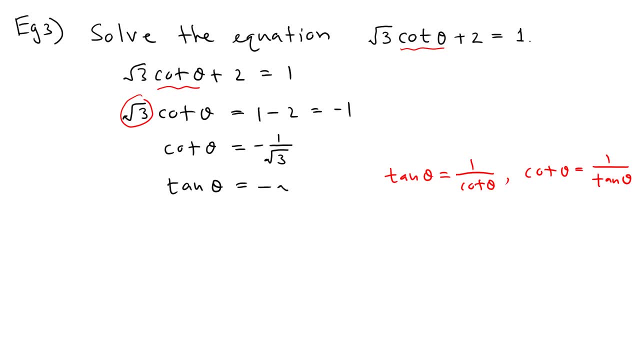 on this side and if you flip this one this can be simply negative square root 3 and then you can see that this is something familiar because it's tangent so now what we're going to do we're going to solve this problem as a tangent problem so now we have tan and then from the astc and you can see it's a tan problem but have a negative sign so that means tan negative means it has to be in the either in the second quadrant or the fourth quadrant so that means tan negative means it has to be in the either in the second quadrant or the fourth quadrant so uh so knowing that then we know how to write the uh two angles so the so the next step now would be to find what is the reference angle so you can find the reference angle so theta r that's a reference angle which is simply ignoring uh so we just ignore the sign we only pick the number here so you can see this is 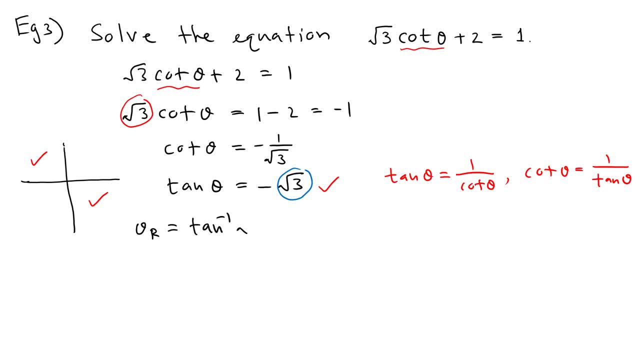 simply tan inverse just the number without the sign and then you can see this is simply coming from the table so tan inverse is equal to three over two that means it is simply pi over three so that is the reference angle but since we deal with uh degrees so you can see instead of uh writing uh radian you can write this the degree value so let's say the degree 60. now since you know the reference angle and then since you know the two quadrant we can write the solution now so that means theta has to be e the since the second quadrant it is b 180. 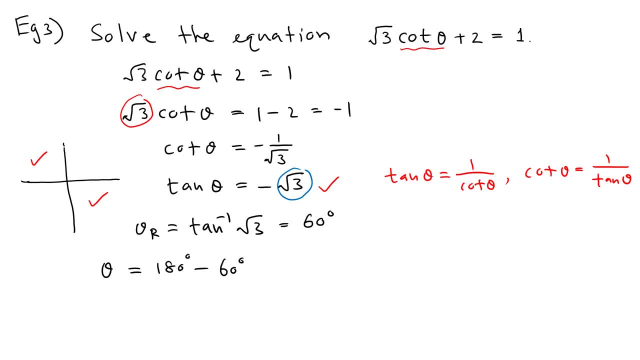 minus 60. that's one in the second quadrant or theta has to be since the fourth quadrant it is 360 minus um 60. that's the reference angle so we subtract the reference angle in this case so this is in at the interval 0 to 360. 360. uh so and if you solve if you 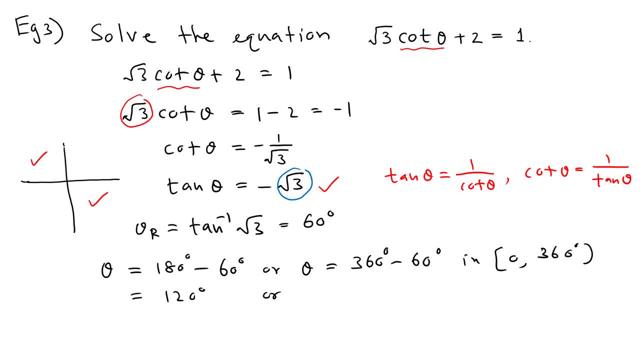 120 here and then oh you're going to get theta equal 300 as the two angles so now we can find the general solution so the general solution the the general solution 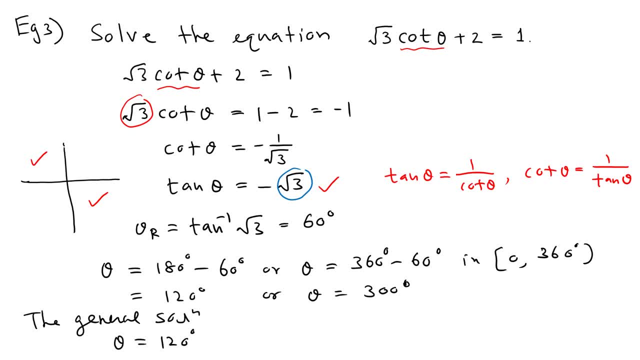 you can write as theta equal 120 plus 360 k o the next one is 100 plus 360 k 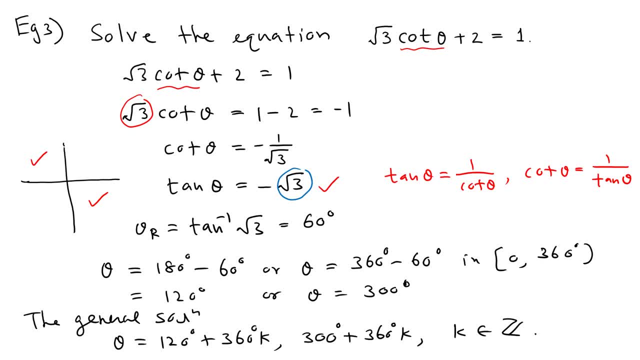 where k is an integer so you can write it like that so that's 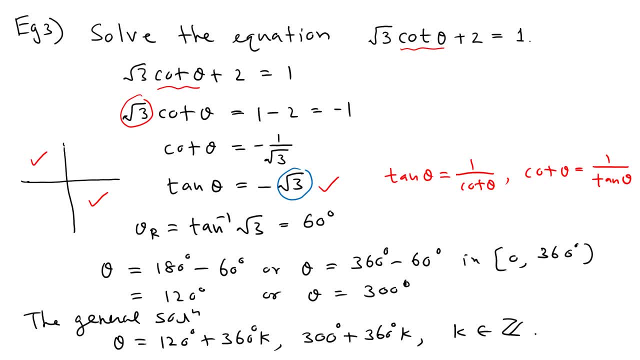 how you solve a problem using uh degrees so here we add multiples of 360. 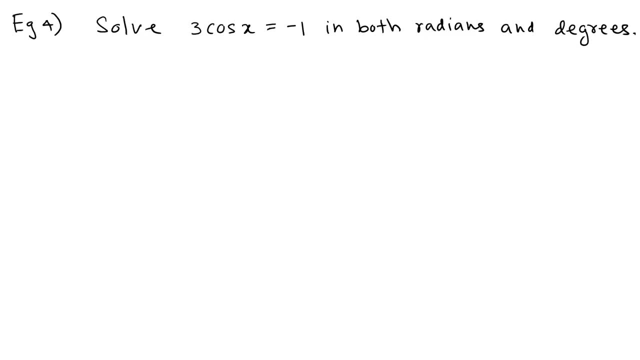 so let's look at the next problem so next we have 3 cosine x equal minus 1 and we're going to solve this a problem in both in radian and decrease so we can isolate the cosine term that's the first step so let's isolate that so we have 3 cosine x equals negative 1 that means cosine x equals negative one third and you will see that this value is not a common value in the cosine table so that means what we can do we can use a calculator uh to find the cosine x and negative one third and you will see that values like we can do approximations you can find exact values we're going to find the approximation approximate values so um and also we notice that this is a cosine and a negative so cosine negative means uh it should be either in the second quadrant or the third quadrant that we noticed 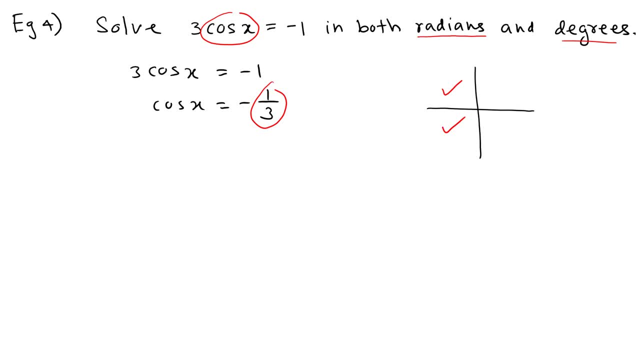 so to find the reference angle what we can do we can ignore the negative sign 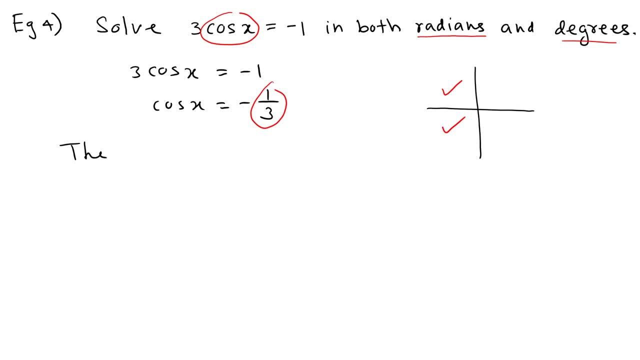 so the reference angle the reference angle 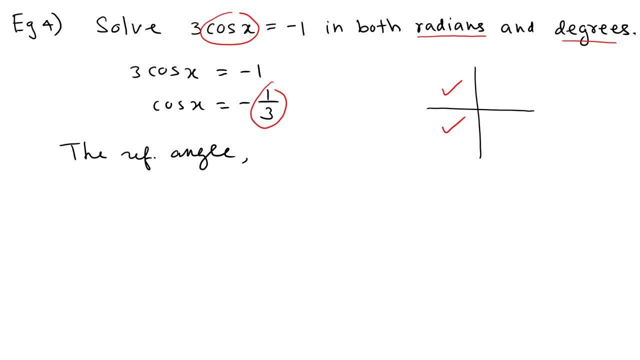 theta r we normally call theta r is simply cosine inverse a one-third we ignore the negative sign and just use the positive value for that and then uh what we can do we can find them in both in the radian and degrees so you have to be careful since uh if the value is small we can't find the negative sign try to write at least three decimal places uh otherwise what will happen when you convert you get a large error and uh your values may not be accurate so uh so we're gonna write the value in radian mode so like if you use a calculator make sure that you turn the model you change the mode to the radian mode and you change the mode to radian and then you find the cosine inverse one-third so you should get one point two three one if you round two three decimal places 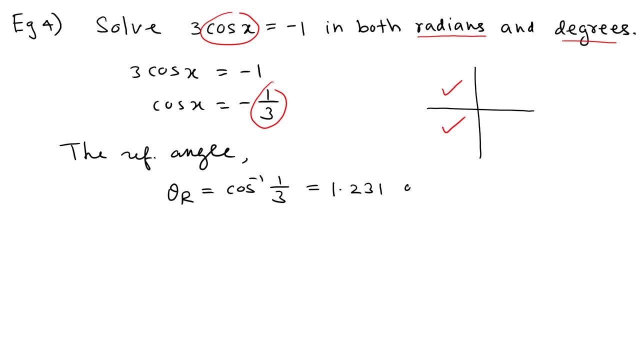 If you round to three decimal places, try to write at least three decimal places. so this is radiant or if you turn the if you turn the mode to the degree and then if you find the value you're going to see that 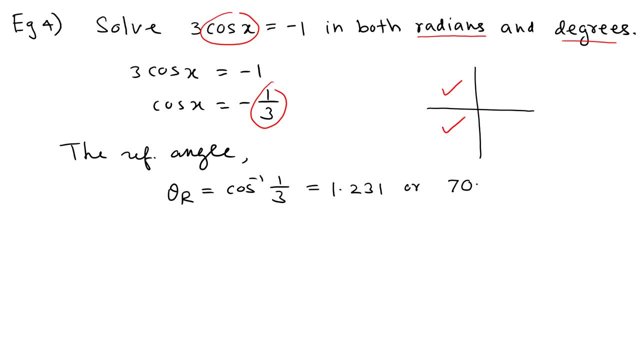 you're going to get 70.53 since this is a larger value we just write only two decimal places so this in degrees 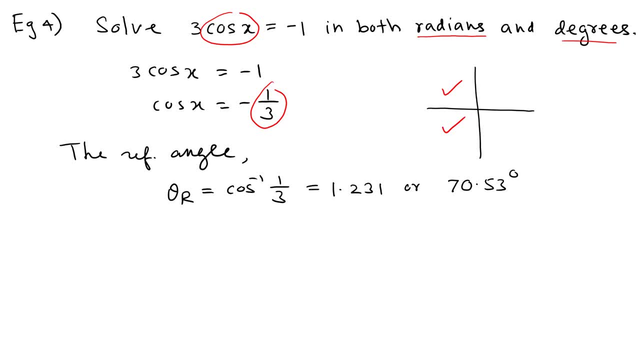 so that difference uh here we are for the radian we write three decimal places because the values are small and for the degrees we really we write only two decimal places but the values are large so that's the 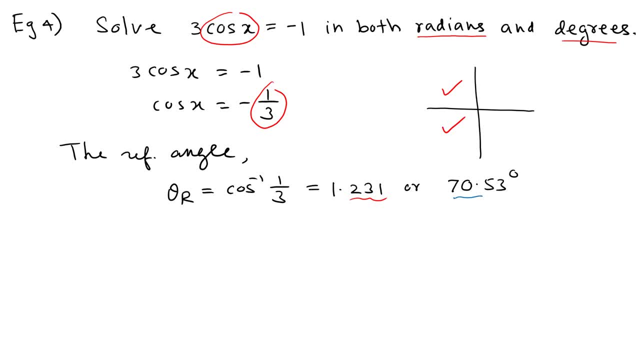 difference so you always need to uh think about that when you solve problems like that otherwise if it's a multiple choice problem you will you will get wrong answers if you if you 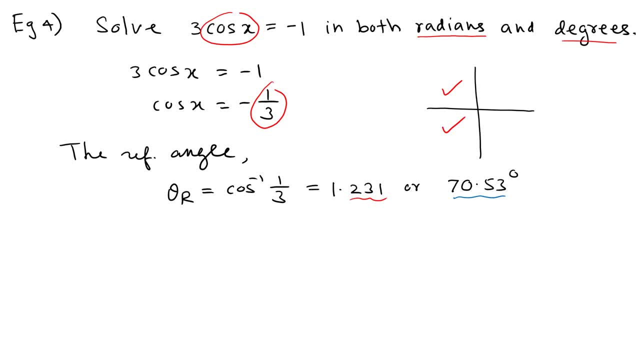 try to convert okay now uh let's try to do this in the uh the degree form uh in the radian form first and see what's gonna happen so these are in the second and third quadrant so in in radian 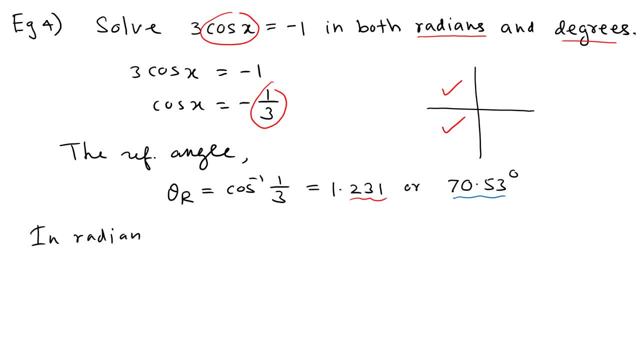 so in in radian you can add two solutions x so in the second quadrant it has to be 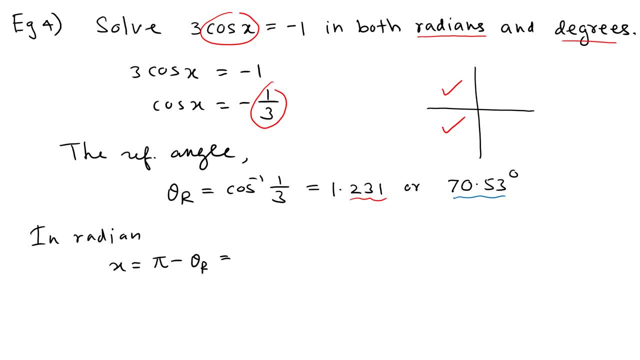 pi minus the reference angle so that means it is pi means 3.142 up to 3 decimal places minus your value is 1.231 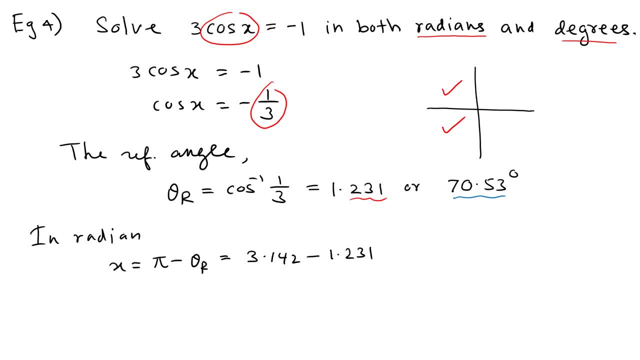 that's the first value um so uh this if you simplify are you gonna get roughly one 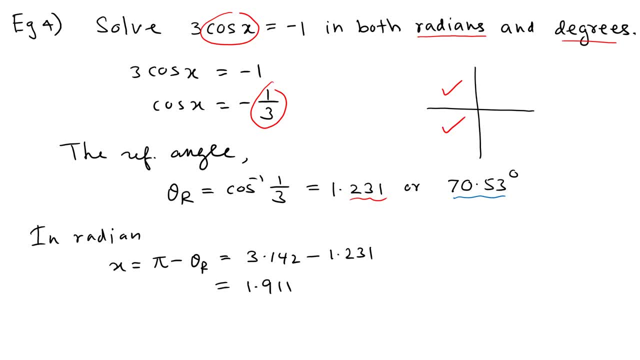 1.911 and then actually let me write okay yes it's 1.911 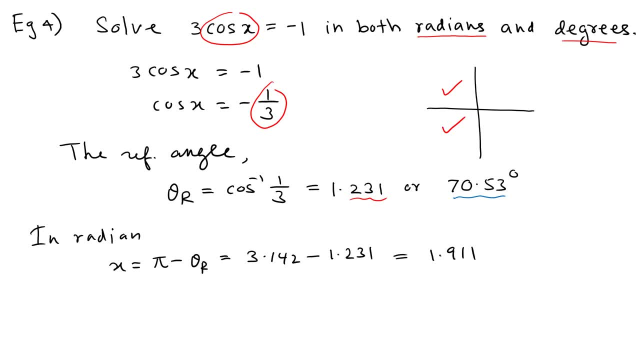 or x equal for the third quadrant it is pi plus theta r so that means 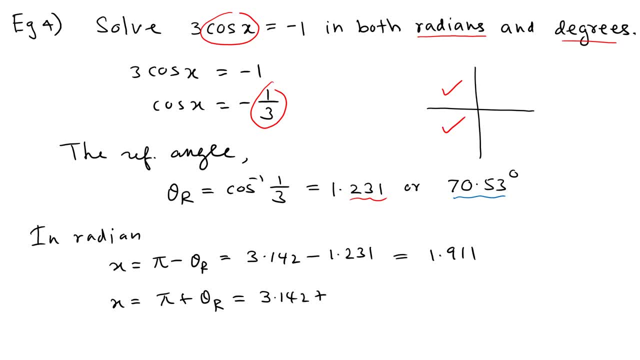 3.142 plus 1.231 and if you simplify you're going to get 4.373 okay now what we can do so this is the 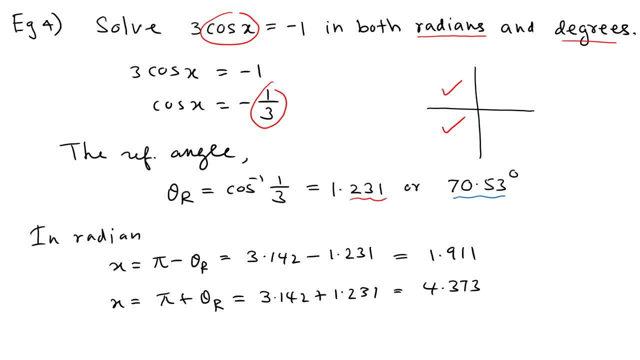 these are the principal values so what we're going to do we're going to add multiples of 2 pi to find the general solution 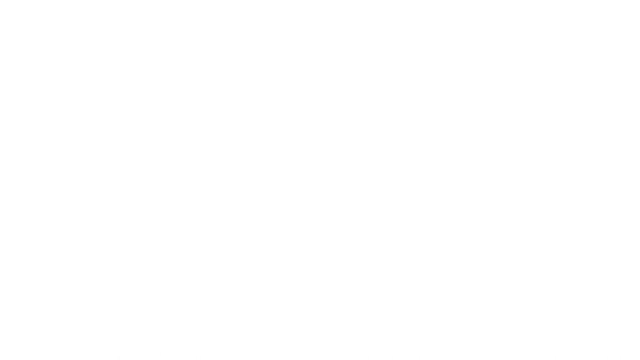 uh so in degree we have so this in degree in degree we can write this one as x equal 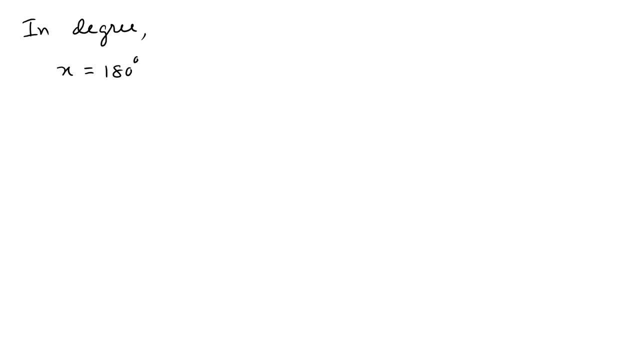 in the second quadrant it is 180 minus 7053 so it simplifies to 109.47 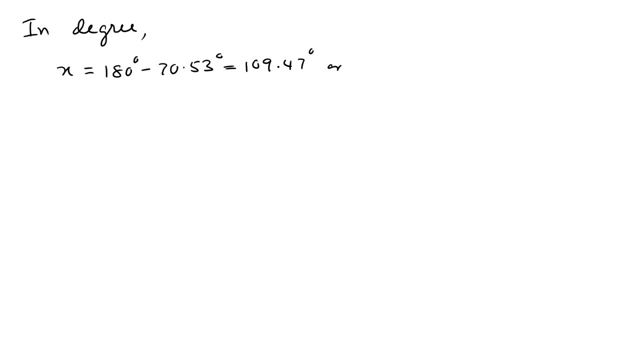 oh and then the other one is x equal 180 plus 7 70.53 so it is 250.3 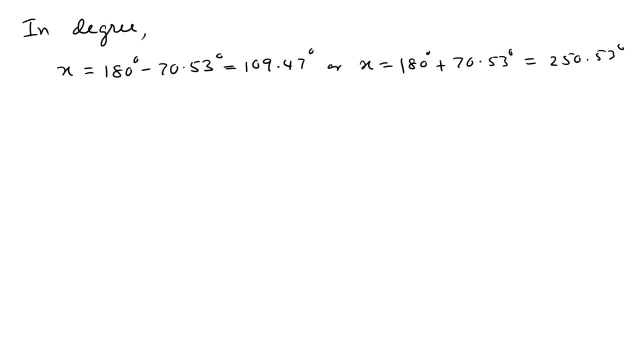 so these approximate values is on exactly these approximate values so the general solution so the general solution in the solution uh in in radian you can write this one as x equal uh 1.911 uh plus two pi k 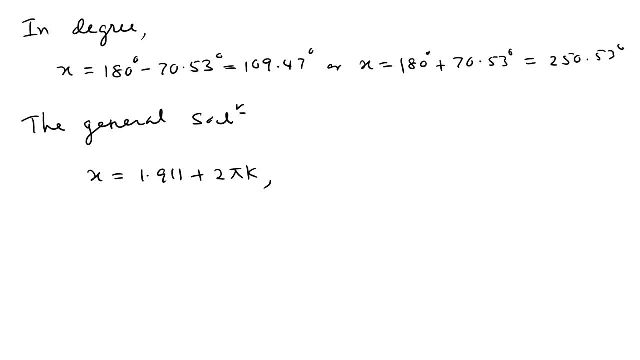 oh x equal 1.911 plus works great 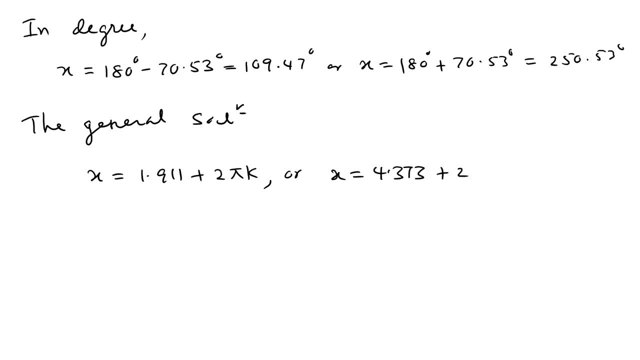 4.373 plus 2 pi k in in degree 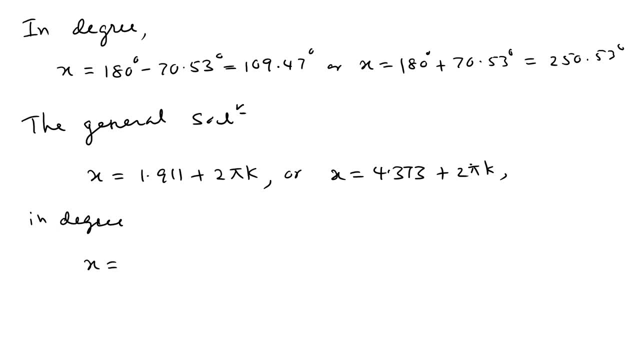 in degrees you can write x equal 109.47 degrees plus 360 k or x equal to 50.53 plus 360 k where k is an integer 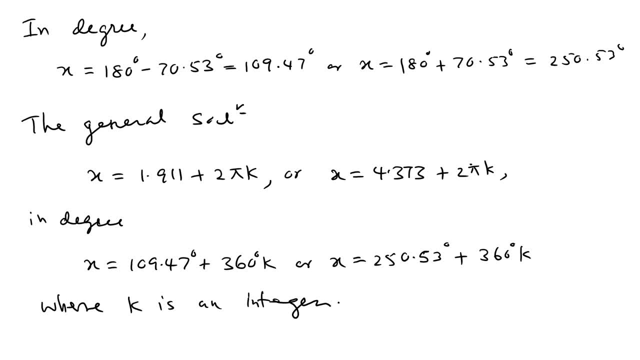 okay so this is how you solve a problem uh where you do not find the uh okay so this is how you solve a problem uh where you do not find the uh where you do not find the uh in the in the table so we just use a calculator and approximate you want to make sure that when you do in in radian if the values are small make sure that you have at least three 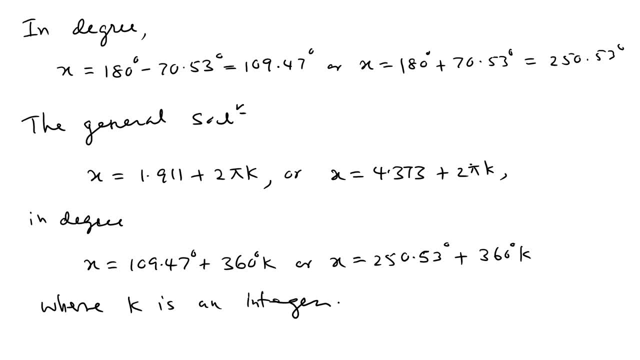 decimal places but in uh if the values are large you uh two additional places are enough so let's look at the next problem 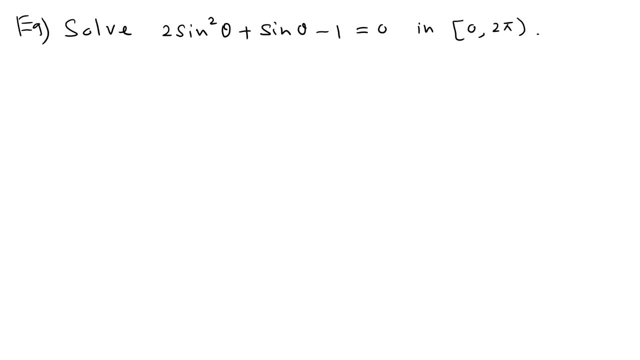 so next we have our two sine square theta plus sine theta minus 1 equals 0 in the interval 0 to 2 pi so we only find the principal values so you can see that this problem is slightly different from 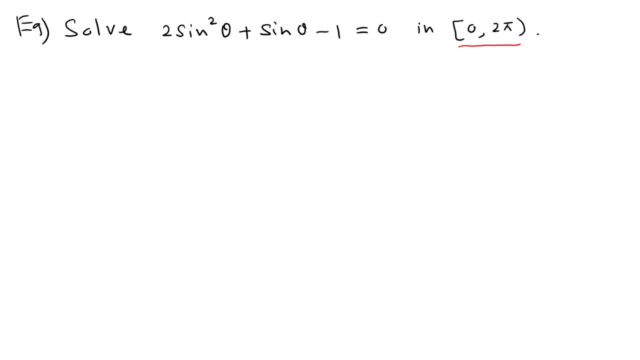 the previous one so since you cannot isolate the sine terms first what we normally do is we're going to factor in a factor so that's the first step uh so that means we can look at the corresponding algebraic equation so if you look at the algebraic equation this looks like 2 x squared plus x minus 1 equals 0 and then we know how to solve a problem like that we can look at the factor factors uh so you're going to look at the the product we're going to multiply these two so you can get negative 2 that means you're going to think of factors uh that's going to give you the product negative 2 and sum 1 so that means you can see that the two numbers are 2 and negative 1 those are two numbers that mean we can directly write the factors so that means uh 2x squared so that means it's going to be 1 has to be 2x the other one has to be x and then the the question is how to get the other numbers so you can see you're going to divide the number by the factorization so we're going to divide 2 we're going to divide the 2 by 2 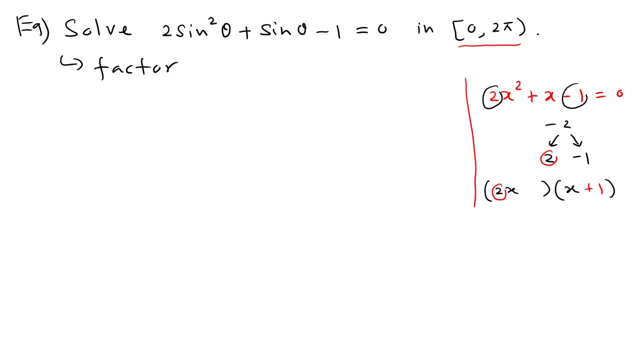 so this should be plus 1 and then we can divide a negative 1 by 1 because that's in front of 1 that means this can be negative 1 that's how we get the two numbers there so that's the factorization so 2x minus 1 x plus 1 that means here x is acting as sine theta so of course because we have this factorization you can simply write this one as 2 sine theta minus 1 that's the first factor the other factor is x plus 1 that means sine theta plus 1 equals 0 so that's what happened uh so after we get the factorization and what we can do is we're going to set each factor equal to 0 so that means for the first one you have 2 sine theta minus 1 equals 0 or sine theta plus 1 equals 0 and from the post-match equation you can see that if you isolate the sine term you can see sine theta is bring 1 to the other side divided by 2 1 half 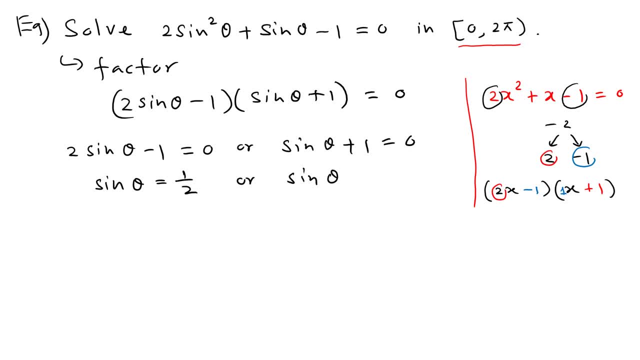 or here we're going to get sine theta equals negative 1 so negative 1 is one of the extreme values so when you have extreme value what we normally do is we can look at the graph so if you look at the graph and you can see that uh so it's a 1 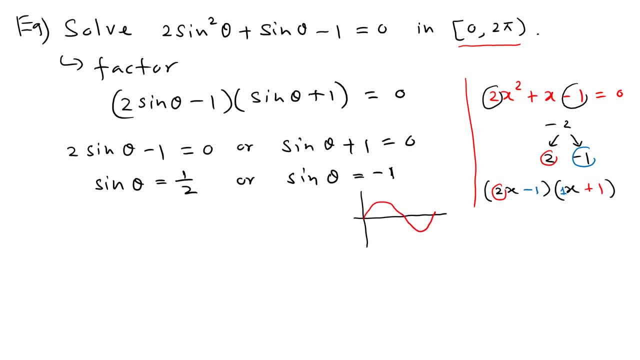 negative 1 and 0 so you can see that uh that's the are the values that you get negative 1 is so that's negative 1 and 1 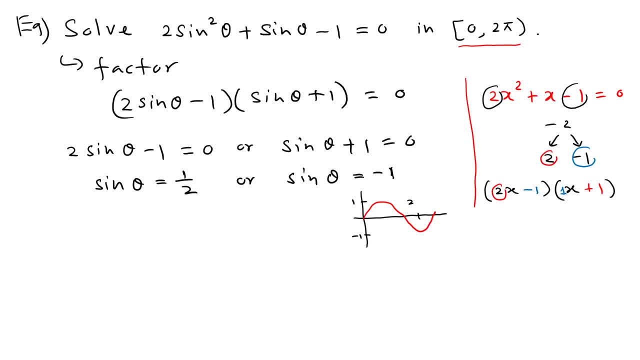 and you can see this value is 3 pi over 2 so 3 times uh so it's a 3 pi over 2 so that's the only value you 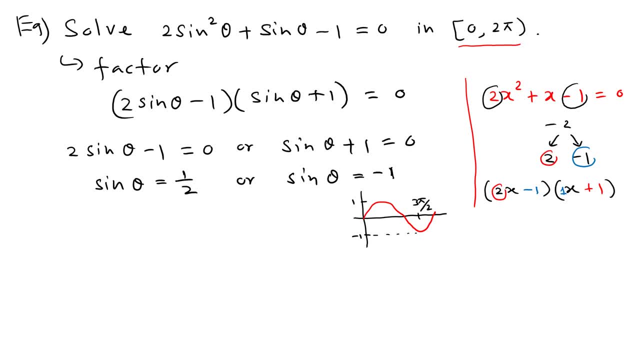 can see there's only one value here there's only one value so you can get that values from the graph so we can use the graph if we need our extreme values what are the extreme values are the zeros and 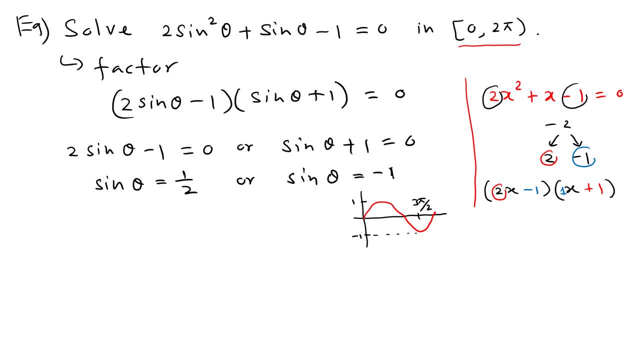 1 over negative 1. so that means for the second equation you can have the solution so it has to be there's only one solution so it is theta equal 3 pi over 2 for the second one we use 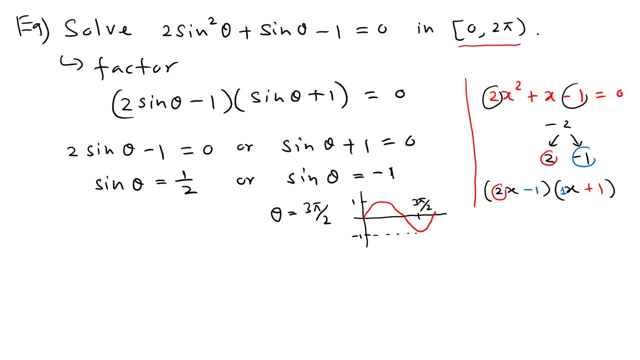 uh we do it as before so we're going to find the reference angle 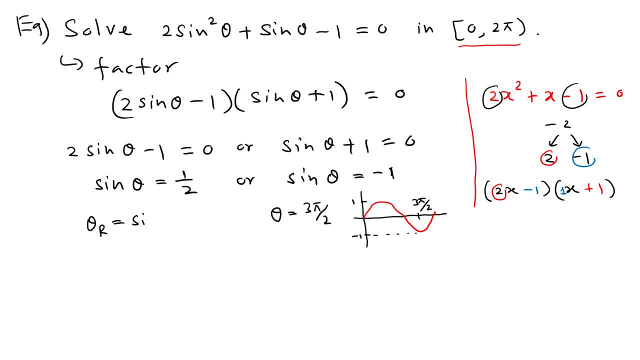 so the reference angle theta r which is sine inverse one half so that means sine one half means is a pi over six and this is positive so since this is positive and you can see that i did that either on the first quadrant or the second quadrant so that means the two values are you can see a theta equal are the first value is one uh one in the first quadrant pi over six and then oh the other value is theta equal pi minus pi over six so which is that's from the second quadrant which is 5 pi over 6. so those are the principal values uh so now uh so we have all three values so we have uh one value we have one value from the second equation and we have two values from the uh first equation i mean we can combine them we normalize them in the increasing order so that means theta equal uh pi over 6 the smallest value and the next one is 5 pi over 6 or 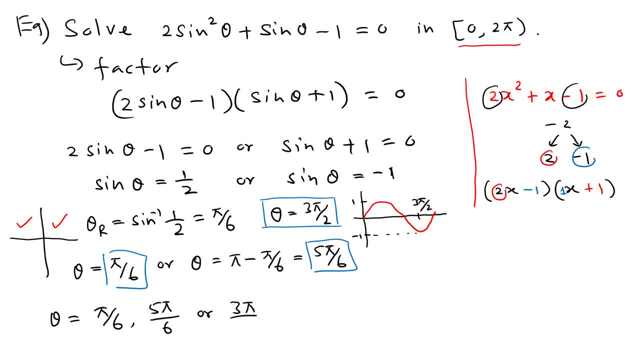 pi over 6 uh 3 pi over 2 in 0 to 2 pi but if in general solutions we simply add the multiples of r 2 pi so that's how we solve the problem so let's look at one more 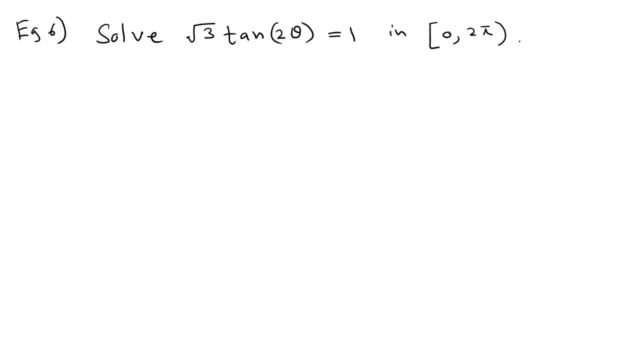 so we have solved square root 3 10 2 theta equal 1 you can see that this problem is different from all the previous problems you can see that this problem is different from all the previous problems 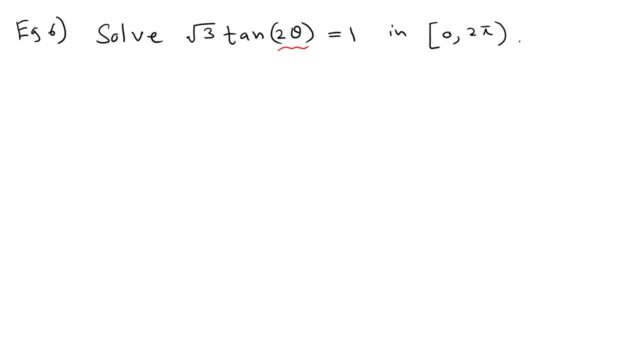 because we have two theta here not theta so that means since we have two theta we want to think about what is the actual range we are looking for because we know that theta has to be in 0 to pi then the 2 theta that means you multiply by 2 is in 0 to 4 pi so that means we first try to solve the equation for 2 theta in the range 0 to 4 pi and then after you do that then we're gonna 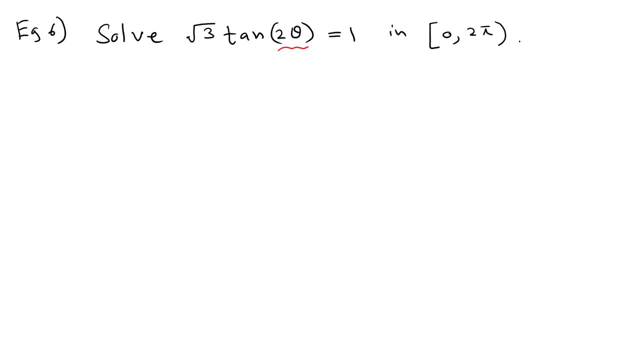 divide by 2 and try to find all the solutions in the range 0 to 2 pi so that means this problem is is completely different from the ones 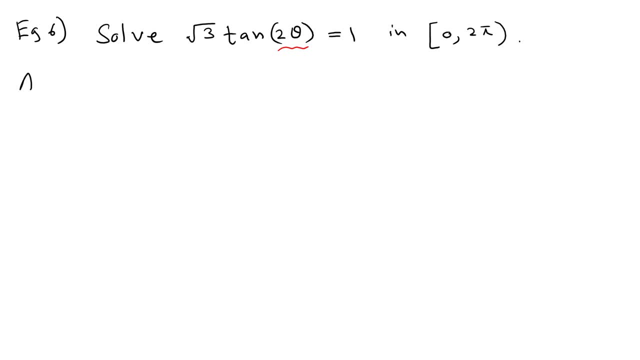 we did earlier so uh so the answer 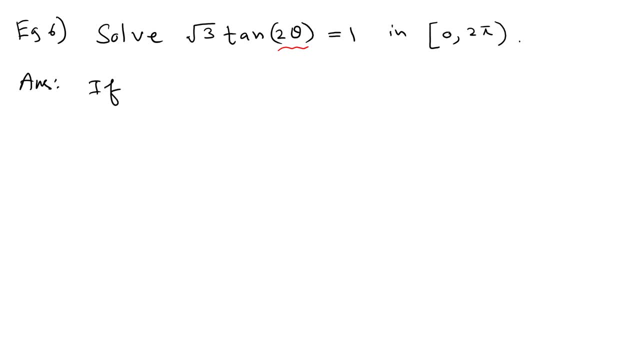 uh so if so let's try this argument if the theta is in uh the interval 0 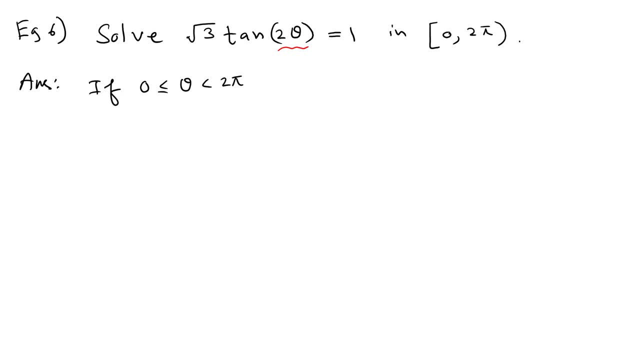 to 2 pi then just multiply by multiply by 2 then 2 theta is in the interval 0 to 4 pi 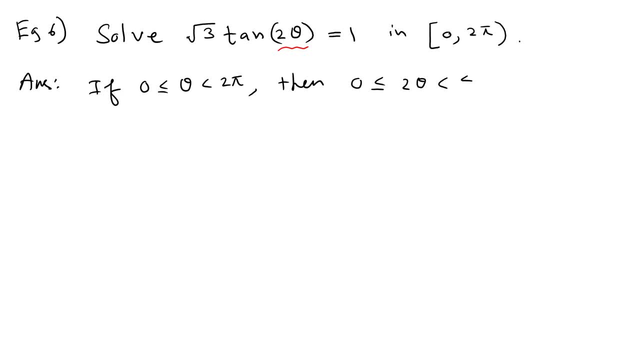 0 to 2 theta 0 to 4 pi so that's we know this so we just multiply by 2 uh both sides when you multiply by 2 you get that so that means what we're trying to do 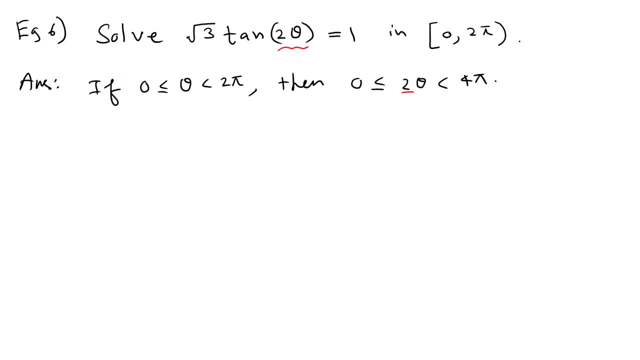 now is we're going to solve this equation for 2 theta not theta but 2 theta that's how we do 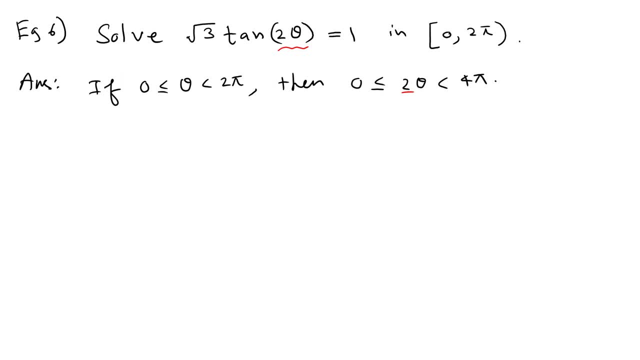 so we just do this as before um so we have square root 3 uh tan theta uh tan 2 theta r equals 1. so that means tan 2 theta 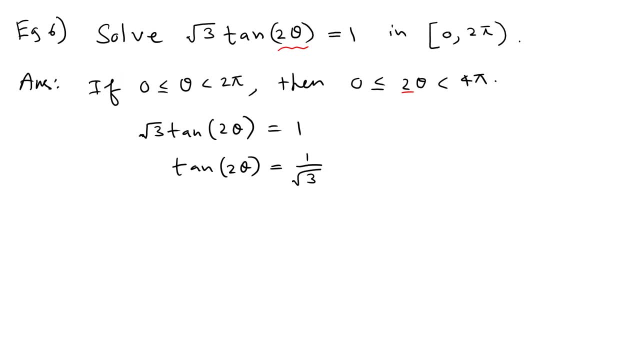 equals 1 over square root 3. so this is like a regular problem for 2 theta and then you can see that again um so this is a tan and positive so that means this angle has to be it in the first quadrant or the third quadrant um so the first 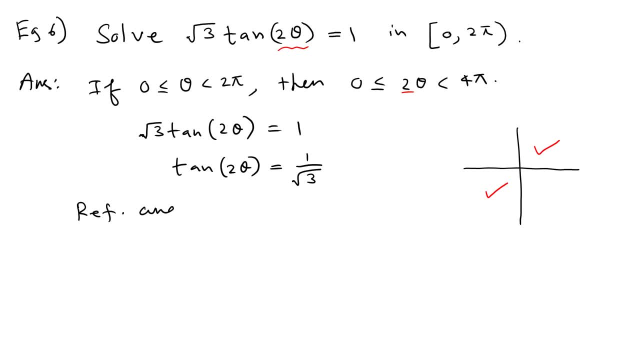 we got the reference angle so the reference angle reference angle theta r which is tan inverse uh 1 over square root 3 so this is simply coming from the table according to the table this has to be pi over 6 so the angle is pi over 6 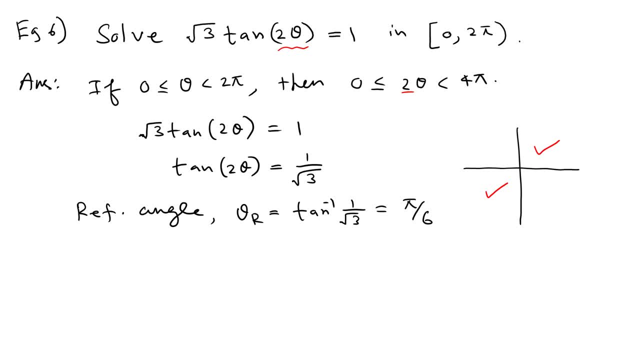 or 30 degrees uh since we know this then we can find the two angles here actually it's not two angles because you can see uh we need to find all the angles from zero to 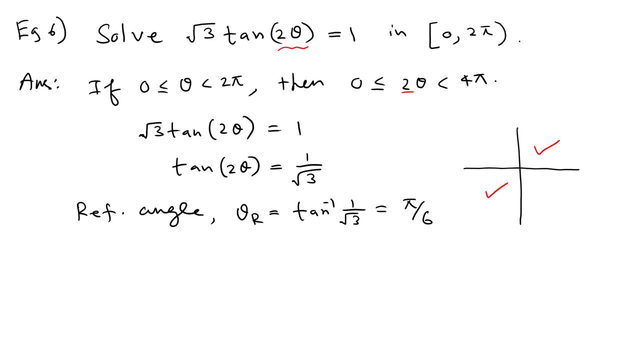 four pi zero to four pi so to to do that so we're gonna so then the two theta is uh pi over six that's the first one and then uh if you add pi so it's a pi so the second angle is actually you can write it like that so the second angle is simply um pi plus 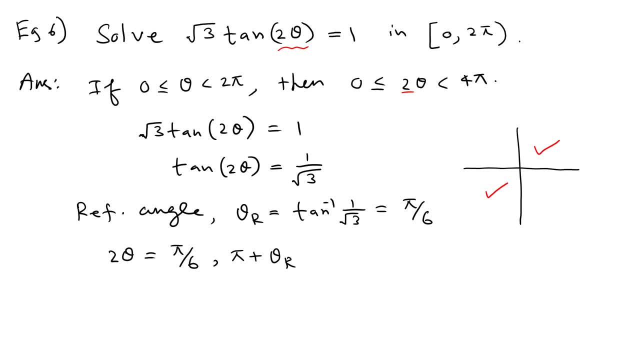 the reference angle that's the uh one in the the third quadrant 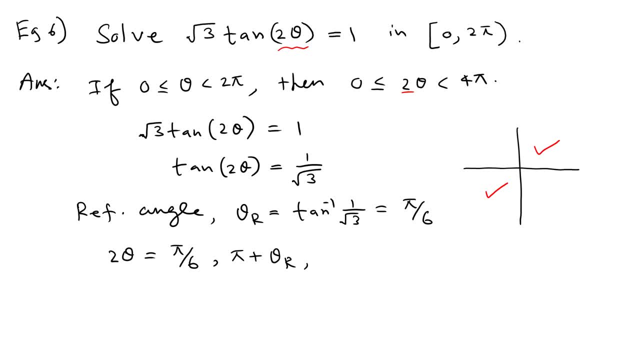 uh and then uh what we're gonna do uh we're gonna add um two pi to these two to get the other two angles because if you go another cycle you get the other angle so that means the next one is pi over six plus a two pi you add one full cycle and then the next one is pi plus theta r again plus two pi so those are the um angles that you can find from zero to four pi because you get one more cycle that's what but that's why i'd be two pi so if you had like a three theta here then you're gonna go two more you're gonna get two more so now if you simplify these so are the angles gonna be pi over six so this one is uh pi plus pi over six and the next one is pi over six plus two pi and then we have pi plus pi over six plus uh two pi so in this case actually you can write 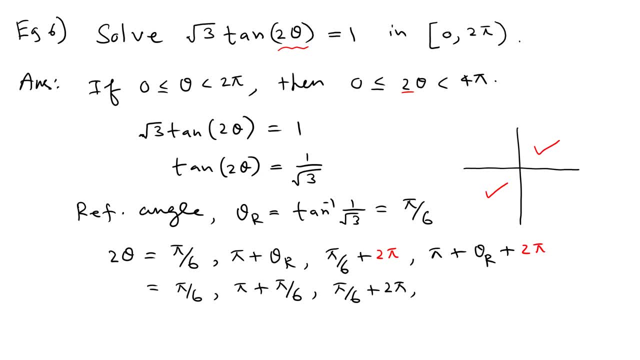 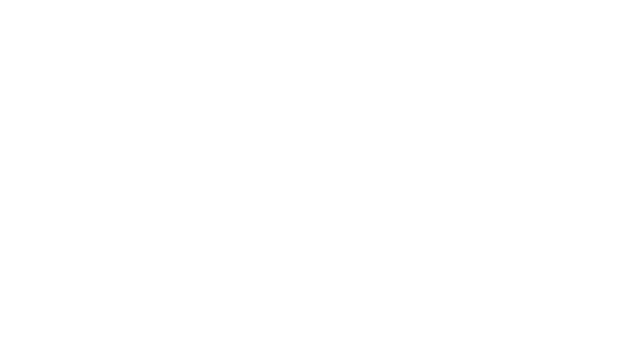 this one as pi over six plus three pi so that's the easy way to write it so you can see pi over six plus three pi so if you simplify and you're gonna get the angles um pi over six that's the first one and this is seven pi over six and then uh we have here uh six times two six times two we have six and two six times two is twelve plus one so thirteen pi so we have thirteen pi over six and the other one is uh six times three eighteen plus one so it's a nineteen uh pi over six so these are the values so this is in uh zero to four pi but what we need we're looking for uh theta that means we're going to divide this one by uh two so that means your final solution you can write like this so you can see dividing by two divided by two you can write theta has to be pi over 12 and then 7 pi over 12 and then 13 pi over 12 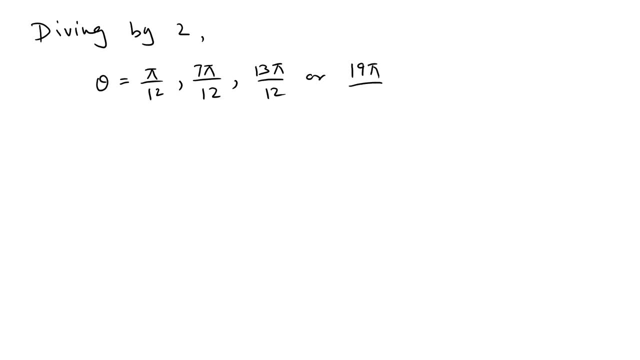 or the final one is 19 pi over 12. so in this case you can see this is again in zero two two pi because we divide by two and if you need the general solution uh you can add multiples of two pi k so you can see if you need a general solution uh that we are we don't need that but i just write the general solution so the general solution general solutions are you can say theta equal pi plus 2 pi k and then 7 pi over 12 plus 2 pi k and then 13 pi over 12 plus 2 pi k and say oh finally you are 19 pi over 12 plus 2 pi k yeah 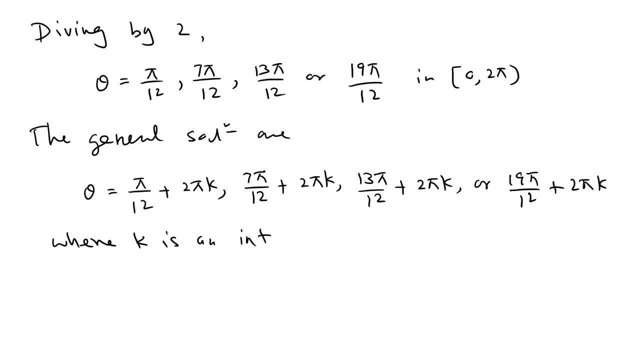 okay is an integer so you can see this problem is slightly different from the previous problem because you have a two theta at the beginning so what we did uh we look uh we multiply the range because we normally know that theta has to be from zero to uh two pi so in uh because of that the two theta is